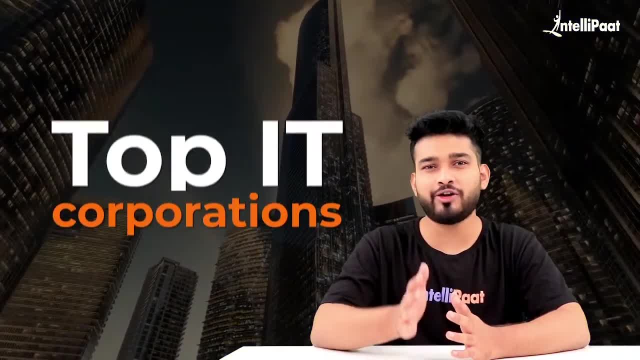 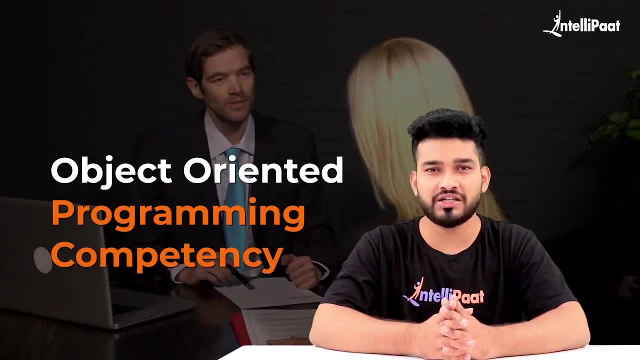 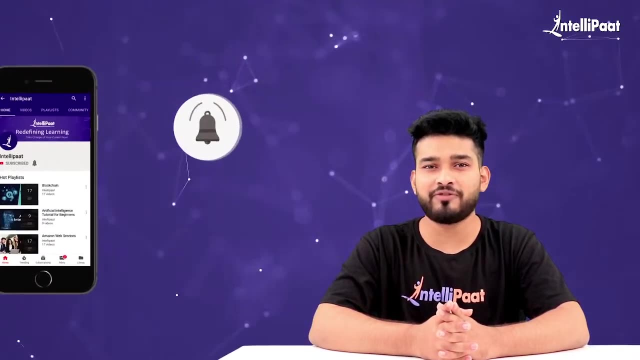 will help you boost your chances of making into the top IT corporations by highlighting top 20 interview questions asked to check object-oriented programming competency. But before we begin this session, make sure you hit that subscribe button so that you never miss an update from Intellipaat. Let's start with a few basic interview questions. 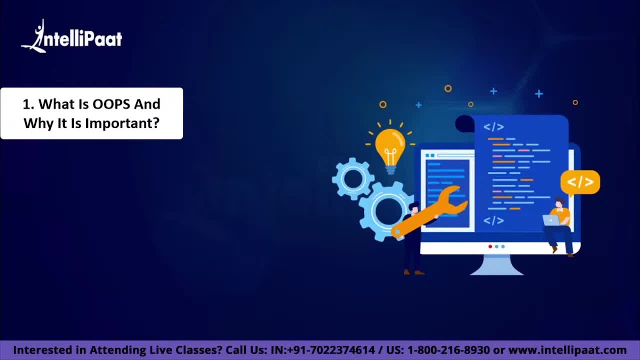 at first. The first commonly asked interview question to the beginners on our list is: what do you understand by the term Oops? why it is important? Now, this is quite basic question, right? But many beginners shatter while formulating an answer to this question, So here is a sample answer to this. 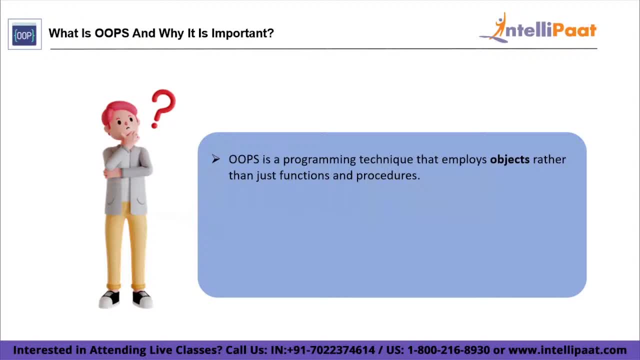 Object Oriented Programming, or OOPS, is a programming technique that relies on objects rather than just functions or procedures. Individual objects are grouped into classes in object oriented programming. OOPS incorporates real world concepts such as inheritance, polymorphism and abstraction into programming. It also enables programmers to encapsulate both data and code together. 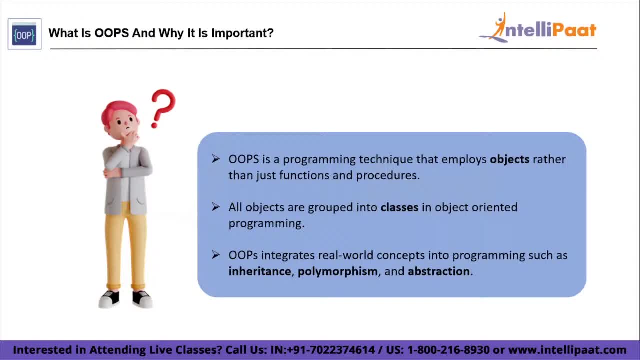 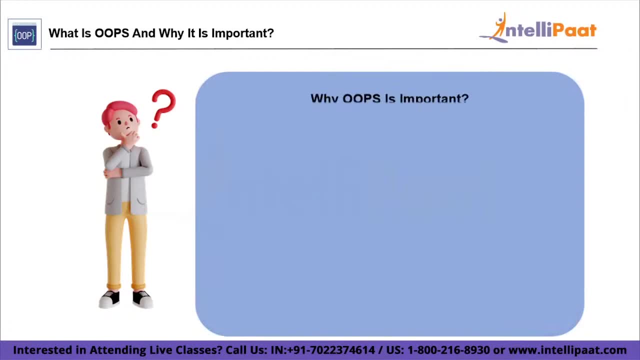 with framework named as class. Now let's move to the second part of our question. That is why OOPS is important. Well, there are plenty of reasons to use OOPS in software development. Let's see a few important ones. OOPS allows more clarity in programming, thereby allowing simplicity in solving complex problems. 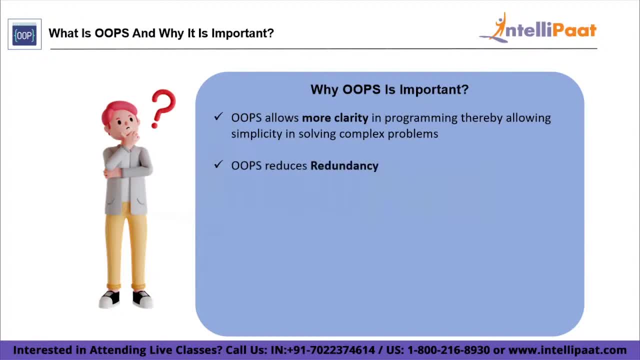 The second one we have is the code developed using classes, and objects can be reused through inheritance. The third important feature of OOPS conveys that Object Oriented Programming provides the ability to sort of bind both data and code together. Also, OOPS allows the data. 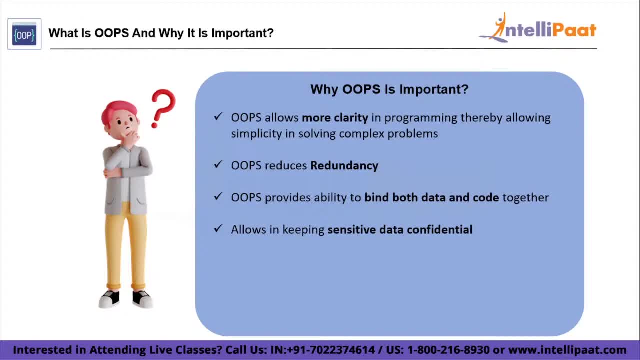 hiding, which enables us to keep sensitive confidential data private from other users. By making use of OOPS, large problems can be divided into smaller chunks, which will definitely improve the code readability. And the last, yet important feature we have is object oriented programming: Object Oriented. 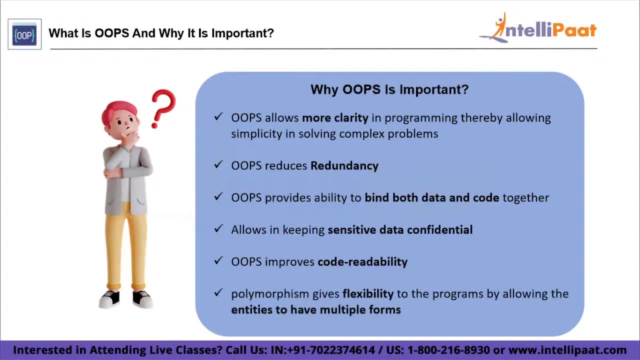 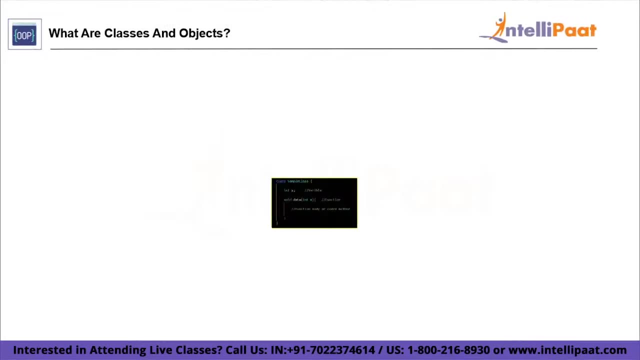 Programming is a concept of polymorphism that gives flexibility to the program by allowing the entities to have multiple forms or multiple functionalities. Let's move to the next question on our list. What do you understand by term class and object? Well, a class is an object's blueprint or template. It is data type that the user specifies. 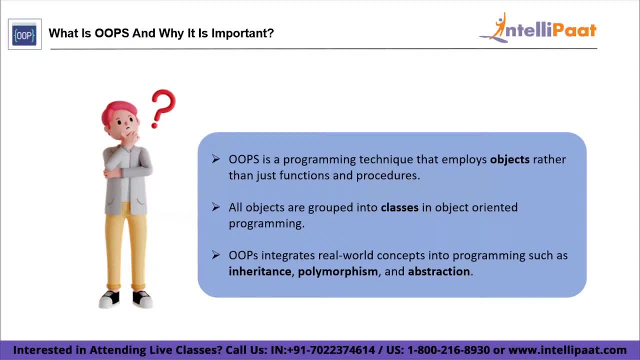 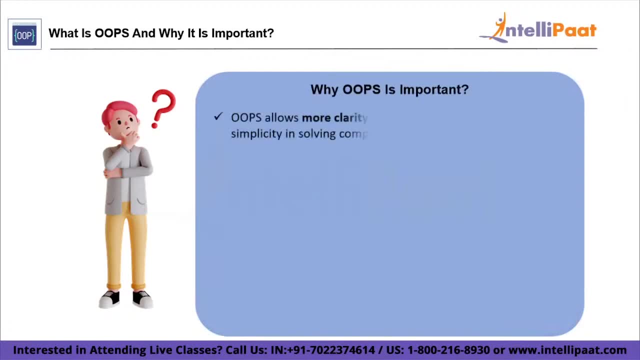 named as class. Now let's move to the second part of our question. That is why Oops is important. Well, there are plenty of reasons to use Oops in software development. Let's see a few important ones. Oops allows more clarity in programming, thereby allowing simplicity in solving complex problems. 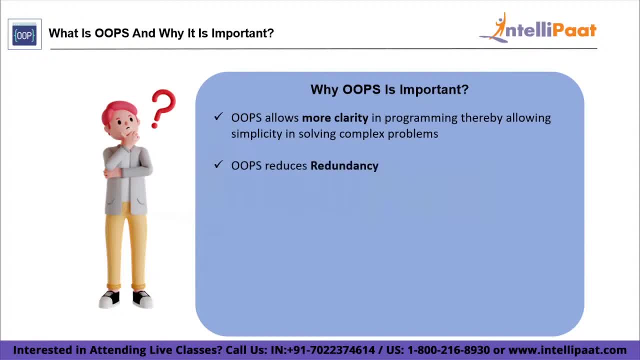 The second one we have is the code developed using classes and objects can be reused through inheritance. The third important feature of Oops conveys that object-oriented programming provides the ability to sort of bind both data and code together. Also, Oops allows the data hiding, which enables us to keep sensitive confidential data private from other users. 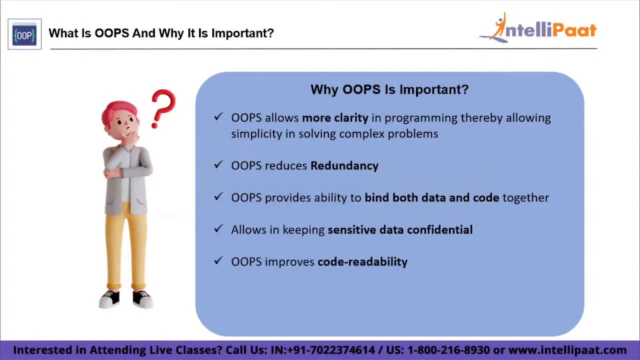 By making use of Oops, large problems can be divided into smaller chunks, which will definitely improve the code readability. And the last, yet important feature we have is that concept of polymorphism gives flexibility to the program by allowing the entities to have multiple forms or multiple functionalities. 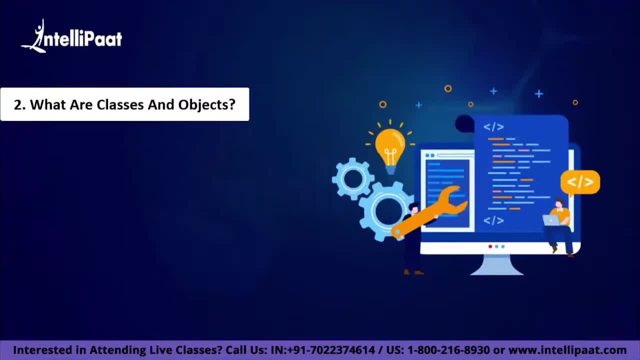 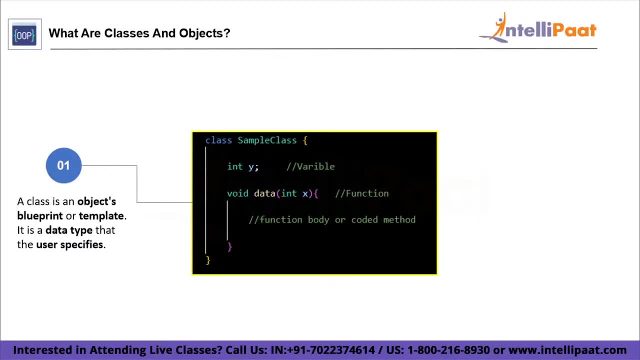 Let's move to the next question on our list. What do you understand by term class and object? Well, a class is an object's blueprint or template. It is data type that the user specifies. Inside it we can define variables, constants, member functions, etc. What I mean by that? 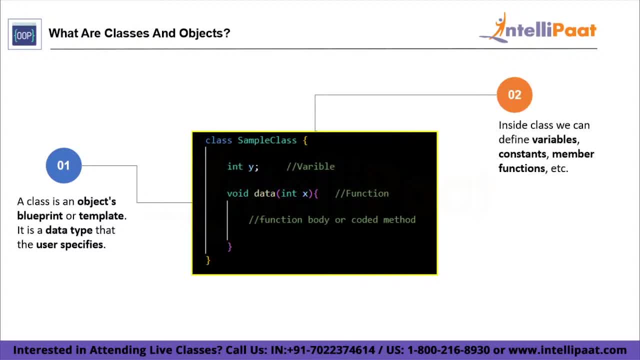 is. When an object is created, it inherits the data that the user has created. It inherits the data that the user has created. It inherits the data that the user has created. It inherits the data and functionalities declared in the class. It does not consume memory at runtime. 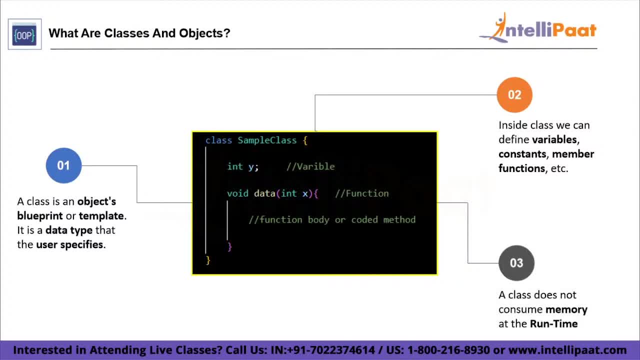 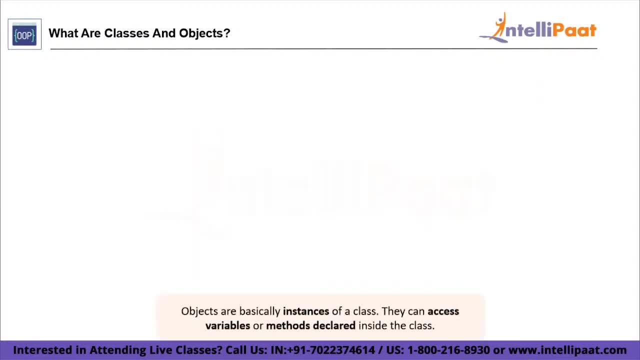 and it just provides the template to the object. Now, if we talk about objects, there are basically instances of classes. They can access variables or methods declared inside the class And, yes, these instances require memory cause. we will be storing both attributes and methods by making use of them. The simple illustration. 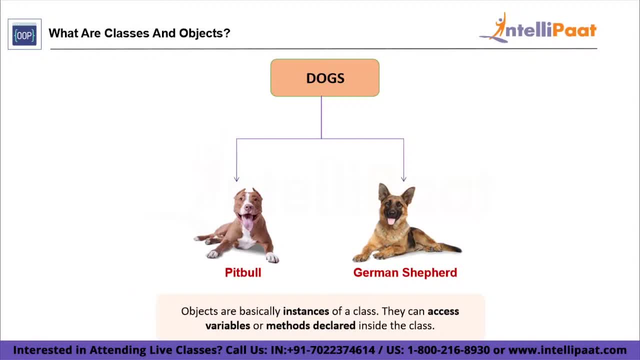 of this would be a dog class. So in the case of dog class, the dog will use the same attributes, attributes and functionalities dogs as an animal possess, And all these properties will be implemented by different breeds, such as Pitbull or German Shepherd. So in programming, oops exactly implements this real-life scenario. 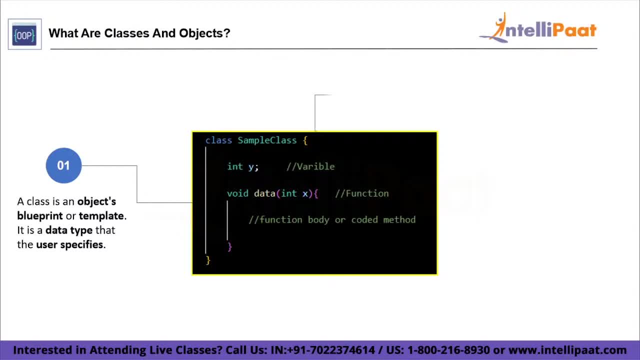 Inside it we can define variables, constants, member functions, etc. What I mean by that is: when an object is created by an object, the object is created by an object. When an object is created by an object, the object is created by an object. When an object is created. 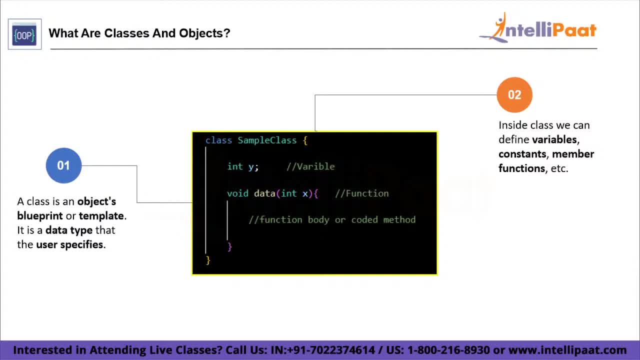 by an object, it inherits the data and functionality declared in the class As in. when an object is created by an object, the object is created by an object. When an object takes the function from the object, it inherits the data and functionality declared in the class. It does not consume. 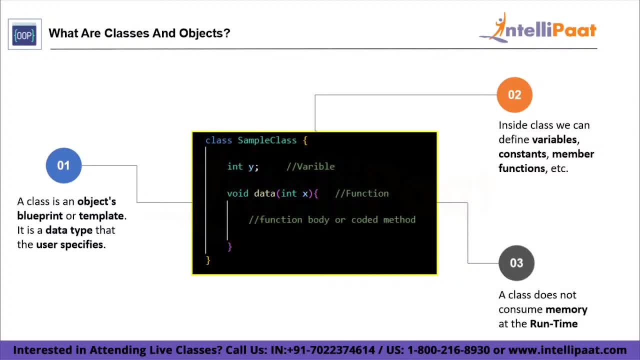 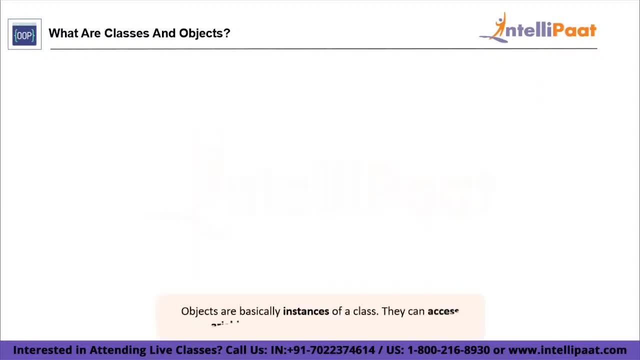 memory at runtime and it just provides the template to the object. Now, if we talk about objects, there are basically instances of classes. They can access variables or methods declared inside the class And, yes, these instances require memory Because we will be storing both attributes and methods by making use of them. The simple illustration. of this would be a dog class. We can also use a dog class, because dog class would be a dog class. I will also mention that we don't use dog class for every sense of the word. However, dog class has only one effect. 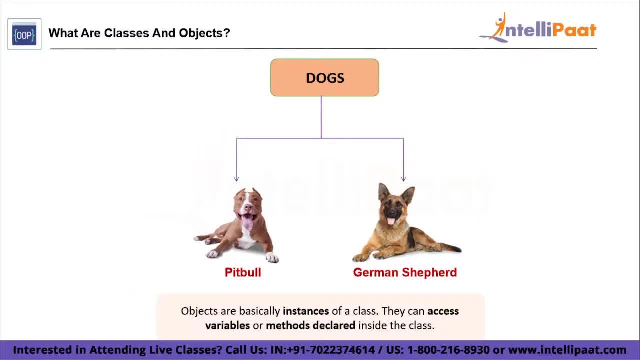 fixed attributes and functionalities. dogs as an animal possess right And all these properties will be implemented by different breeds, such as Pitbull or German Shepherd right. So in programming, OOPS exactly implements this real-life scenario for problem solving. The third question we have is: what do you understand by term pure object-oriented programming? 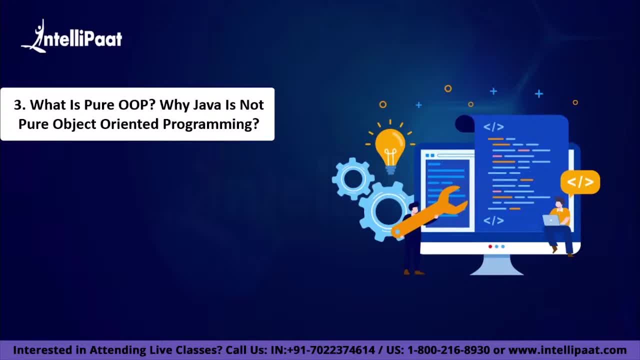 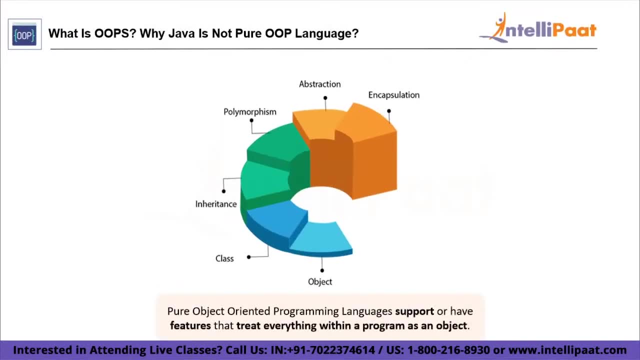 and why Java is not considered as pure object-oriented programming language. Well, a pure object-oriented language's support, or have features which treat everything inside a program as an object. These languages must abide by all the properties of object-oriented programming paradigm, such as encapsulation, inheritance, polymorphism, abstraction. furthermore, all predefined or 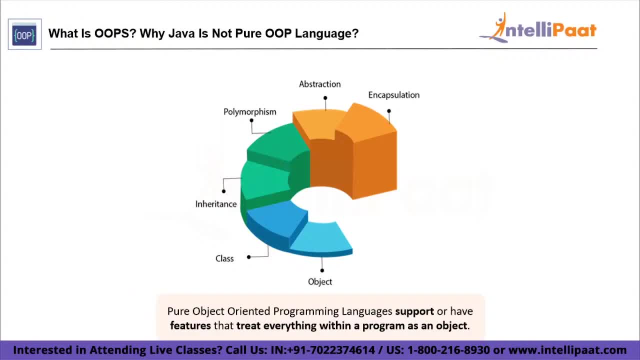 user-defined types in these languages will be objects. there will be no primitive data type such as integer, float or character, And that's where Java fails pretty much. Java allows it to understand features of object and object, but it shouldn't challenge it. 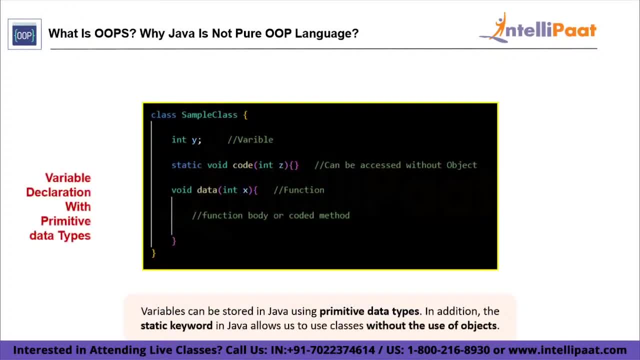 Java allows it to understand features of object and object, but it shouldn't challenge it. Java allows it to understand features of object and object, but it shouldn't challenge it. Java allows allows storage of variables using primitive data types. Also, we have static keyword in. 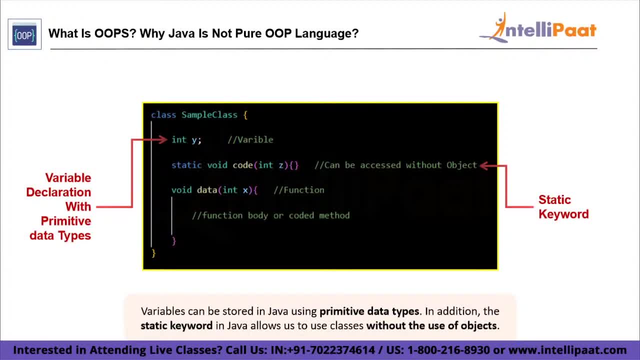 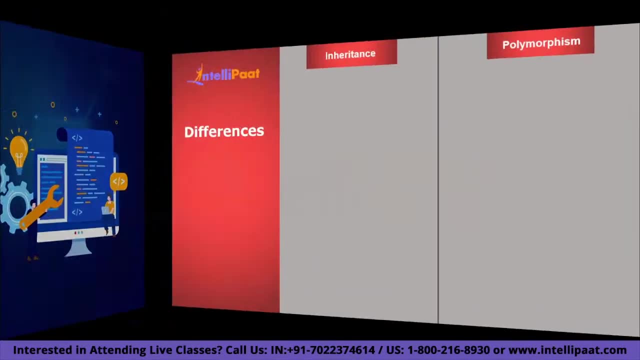 Java, which allows us to use classes without the use of object. That is why Java is not considered a 100% pure object-oriented programming language. Now that brings us to the fourth question on our list: What are the differences between inheritance and polymorphism? Inheritance is one in which a derived class inherits the 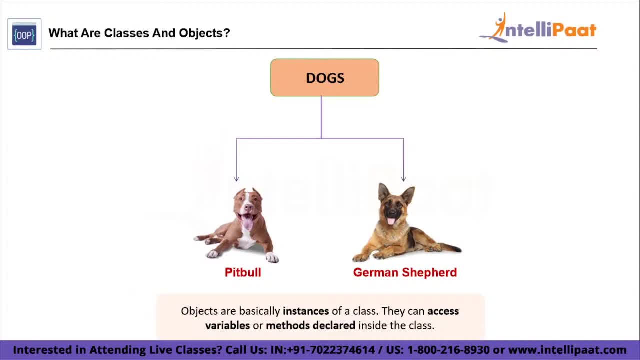 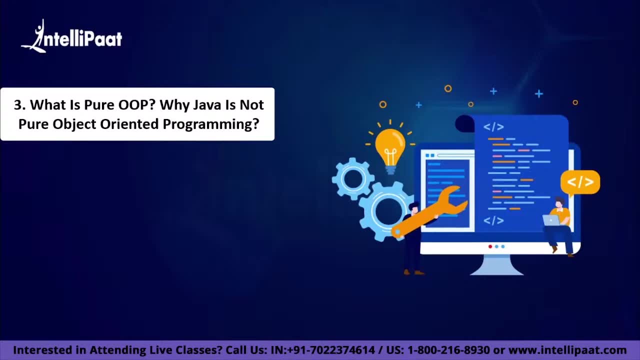 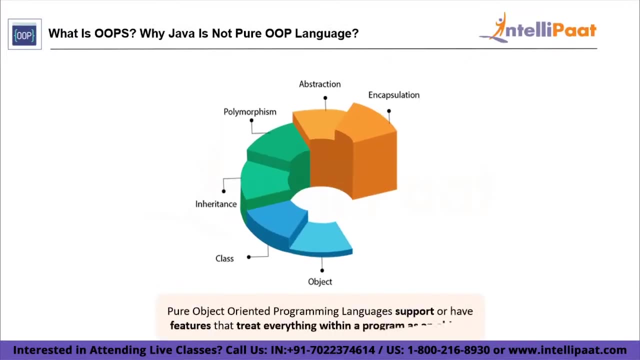 for problem solving. The third question we have is what do you understand by term pure object-oriented programming and why Java is not considered as a pure object-oriented programming language. Well, a pure object-oriented languages support or have features which treat everything inside a program as an object. 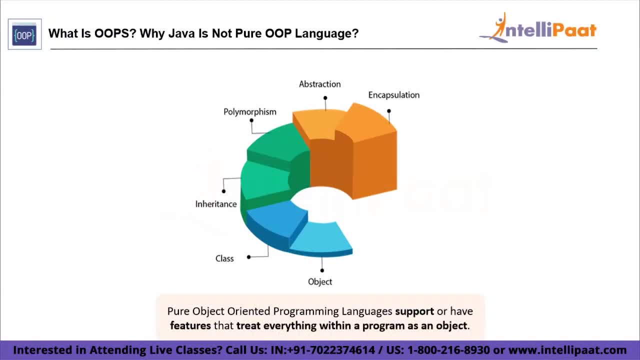 These languages must abide by all the properties of object-oriented programming paradigm, such as encapsulation, inheritance, polymorphism, abstraction. Furthermore, all predefined or user-defined types in these languages will be objects. There will be no primitive data types such as integer, float or character, And that's where Java fails pretty much. 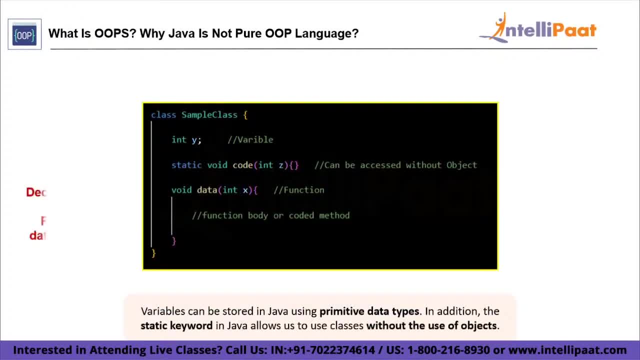 Java allows storage of variables using primitive data types. Also, we have static keyword in Java, which allows us to use classes without the use of object. That is why Java is not considered a 100% pure object-oriented programming language. Now that brings us to the fourth question on our list: What are the differences between? 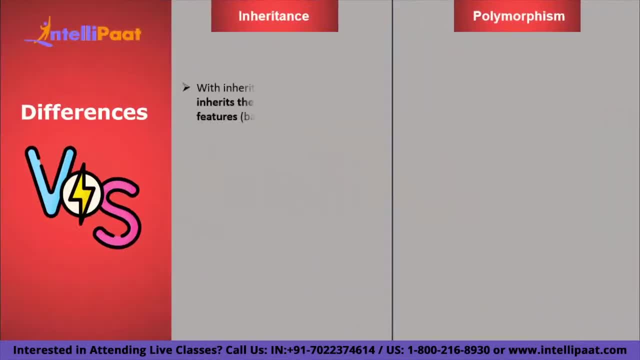 inheritance and polymorphism. Inheritance is one in which a derived class inherits the already existing class future, Whereas inheritance is one in which a derived class inherits the already existing class future, Whereas inheritance is one in which a derived class inherits the already existing class future. 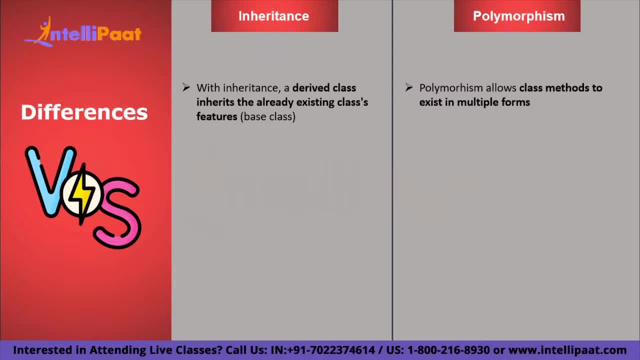 Whereas polymorphism is one that you can define an existence of a class method in multiple forms. Inheritance refers to using the structure and behavior of a parent class in subclass. On the contrary, polymorphism intends on changing the behavior of parent or superclasses method. 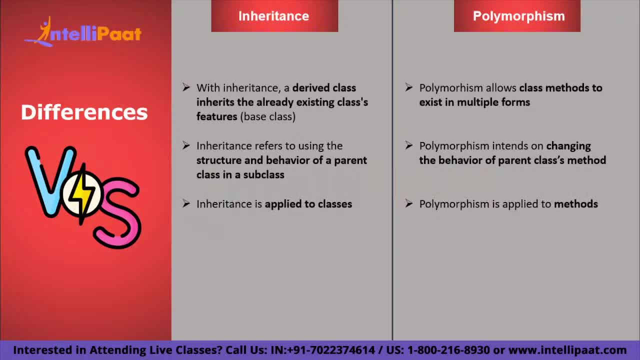 Inheritance is applied to classes And it is pretty clear that polymorphism is applied to methods. Inheritance can be single, hybrid, multiple hierarchical multipath and multilevel types. On the other hand, polymorphism can be single, hybrid, multiple hierarchical multipath. 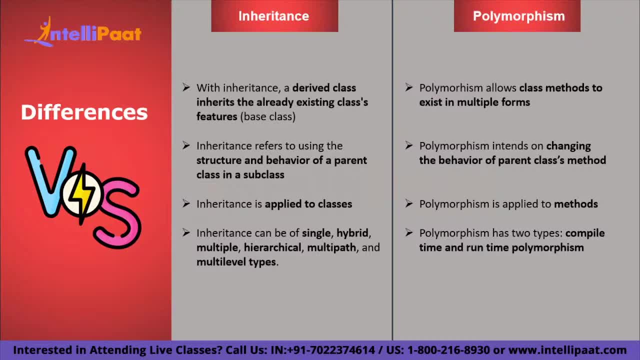 and multilevel types. Polymorphism can be single, hybrid, multiple hierarchical, multipath and multilevel types. The polymorphism has just two types: compile time and runtime. polymorphism- Inheritance- supports code reusability and reduces lines of code, whereas the polymorphism 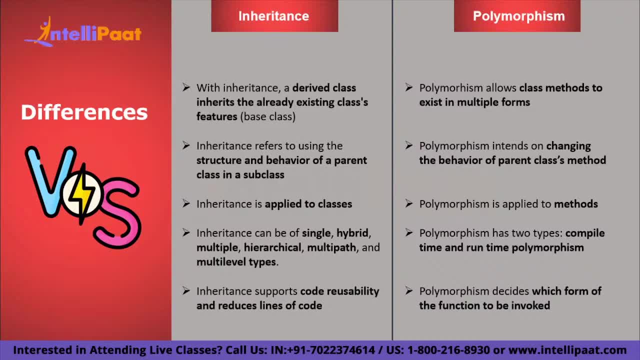 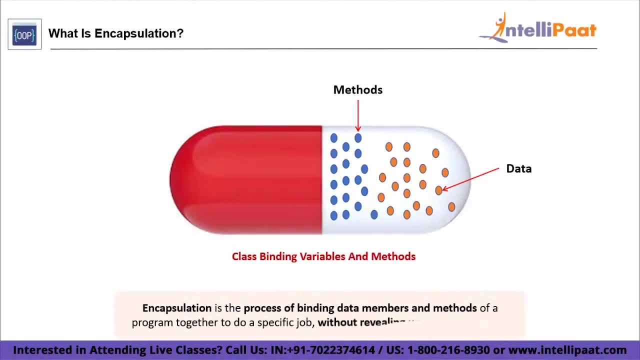 decides which form of function to be invoked. Inheritance supports code reusability and reduces lines of code, whereas the polymorphism decides which form of function to be invoked. Next question we have is: what is encapsulation? Encapsulation can be visualized as the process of placing everything needed to complete the 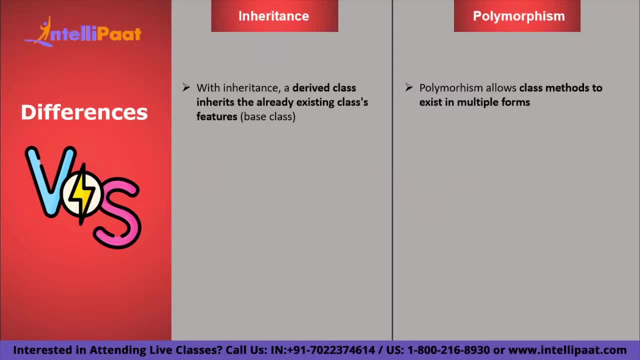 already existing class future, whereas polymorphism is one that you can define an existence of a class method in multiple forms. Inheritance refers to using the structure and behavior of a parent class in subclass. On the contrary, polymorphism intends on changing the behavior. 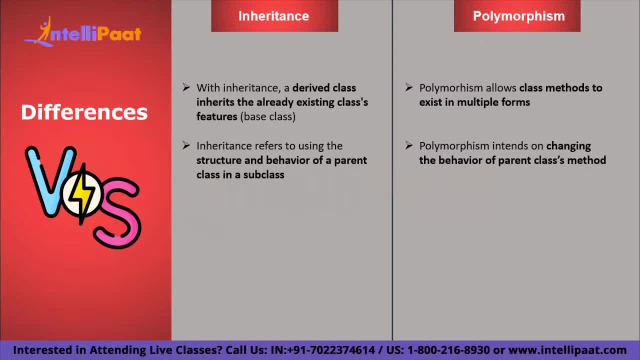 of parent or superclasses. method Inheritance is applied to classes and it is pretty clear that polymorphism is applied to methods. Inheritance can be single, hybrid, multiple, hierarchical multipart or binary. Inheritance can be single, hybrid, multiple, hierarchical multipart. 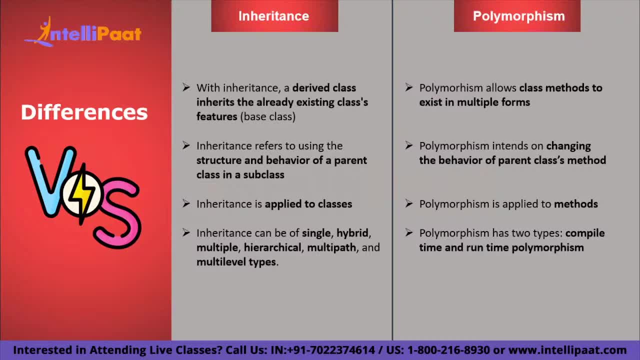 and multi-level types. On the other hand, polymorphism has just two types: compile-time and runtime. polymorphism- Inheritance- supports code reusability and reduces lines of code, whereas the polymorphism decides which form of function to be invoked. Next question we have is: what is encapsulation? Encapsulation can be visualized as the process. 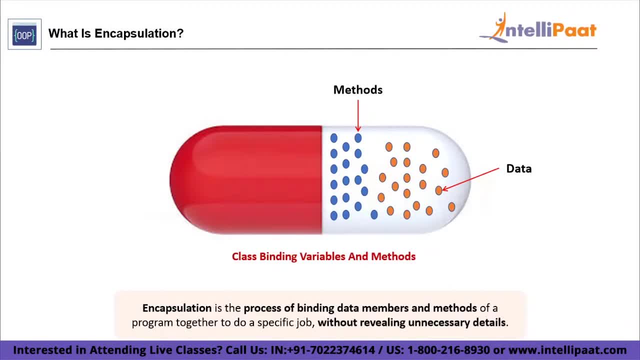 of placing everything needed to complete the work within a capsule and giving that capsule to the user. Encapsulation means that all relevant components, all relevant data and operations are bound together and all the unnecessary details are hidden to the normal user. Encapsulation is actually a technique of tying data members. 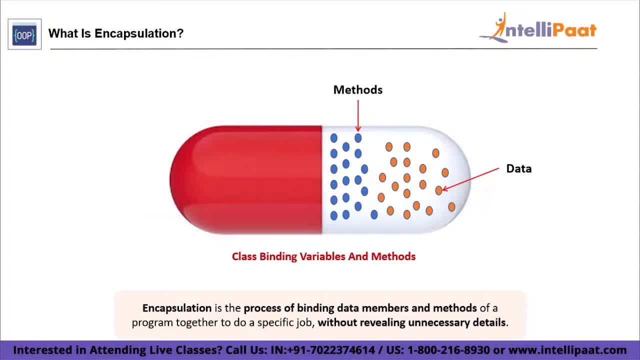 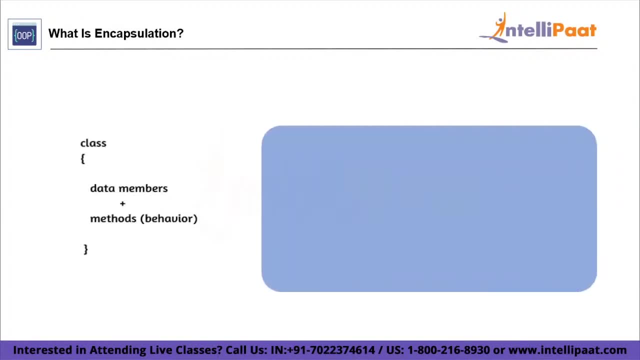 and methods of a program together to execute a specified purpose without disclosing unnecessary details. It can also be defined in two different ways: data hiding and data binding. Data hiding because encapsulation is the process of hiding unwanted information, such as restricting access to any member of an object. Incapsulation is the process of hiding unwanted information. 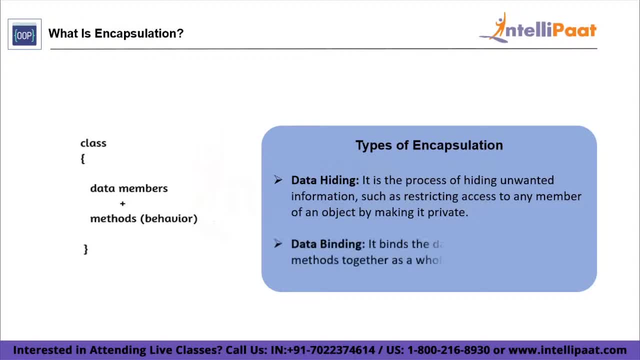 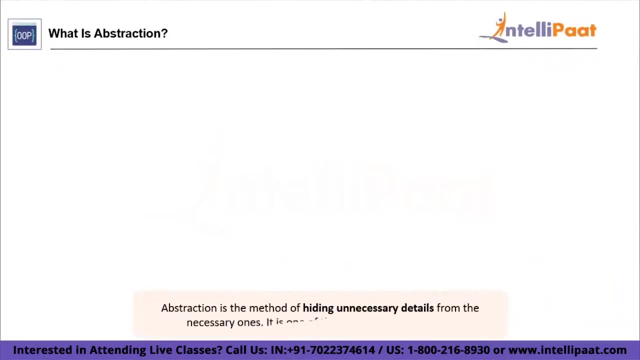 such as restricting access to any member of an object by making it private and data binding, as it binds the data, members and the methods together as a whole, as a class to be precise. Now that brings us to the next question on our list: what is abstraction If you are a user and you have a problem statement? 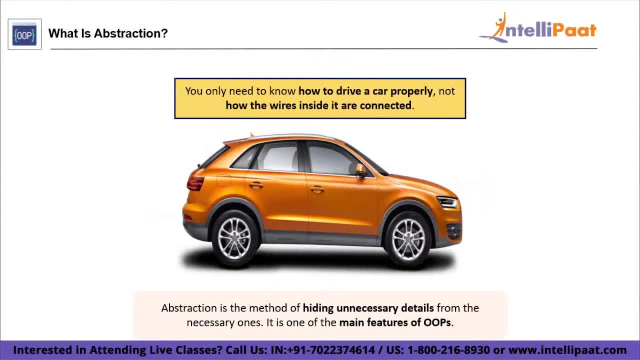 you don't want to know how the components of the software work or how it's made right. You only want to know how the software solves your problem. Abstraction is the method of hiding unnecessary details from the necessary ones. It is one of the main features of object-oriented programming. For example, consider a car. 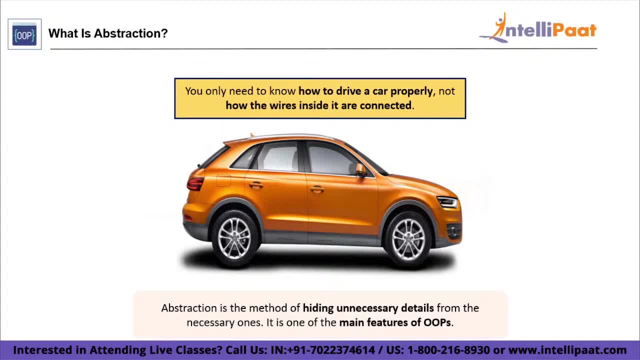 If you want to drive a car, you don't need to know how the wires in the car are connected, right, And that is unnecessary detail for you. you just need to know how to drive a car, and that is the exact process abstraction gives us. Now moving ahead, we'll explore. 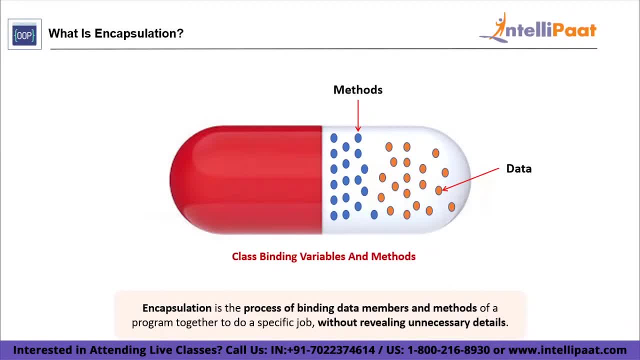 work within a capsule and giving that capsule to the user. Encapsulation means that all relevant data and operations are bound together and all the unnecessary details are hidden to the normal user. Encapsulation is actually a technique of tying data, members and methods of a program together. 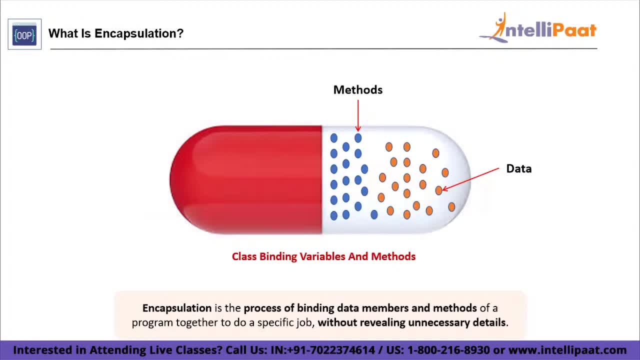 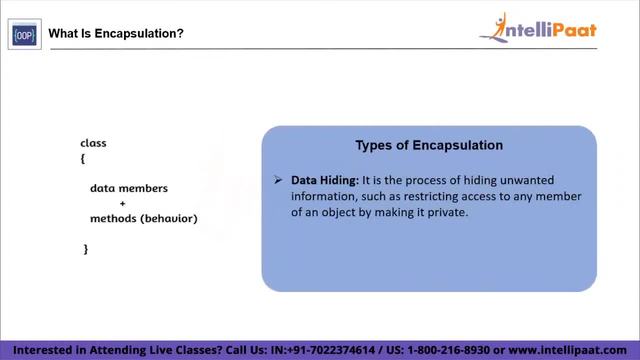 to execute a specified purpose without disclosing unnecessary details. It can also be defined in two different ways: data hiding and data binding. Data hiding, because encapsulation is the process of hiding unwanted information, such as restricting access to any member of an object by making it private. 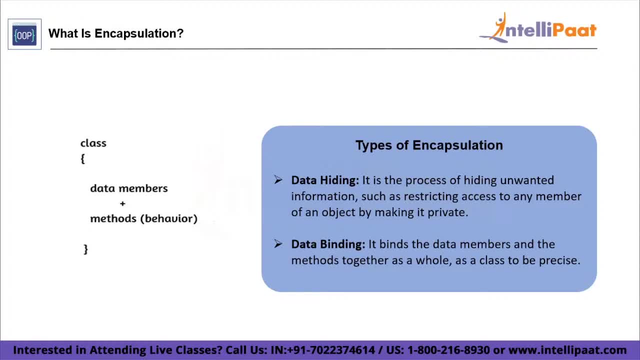 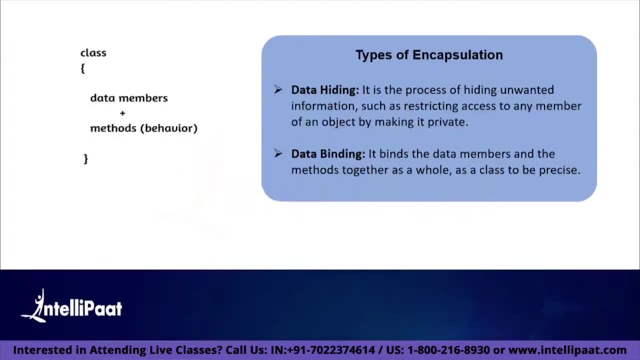 and data binding, as it binds the data, members and the methods together as a whole, as a class to be precise. Now that brings us to the next question on our list: What is abstraction If you are a user and you have a problem statement? 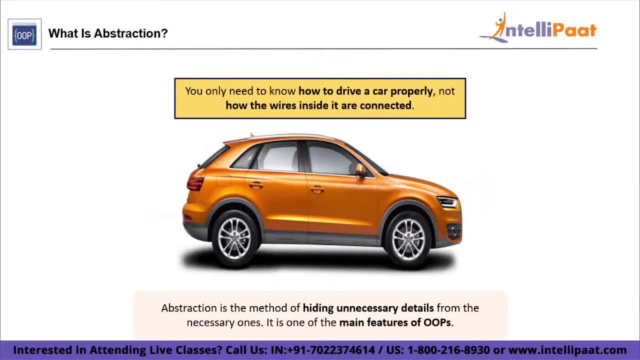 you don't want to know how the components of the software work or how it's made right. You only want to know how the software solves your problem. Abstraction is the method of hiding unnecessary details from the necessary ones. It is one of the main features of objectivity. 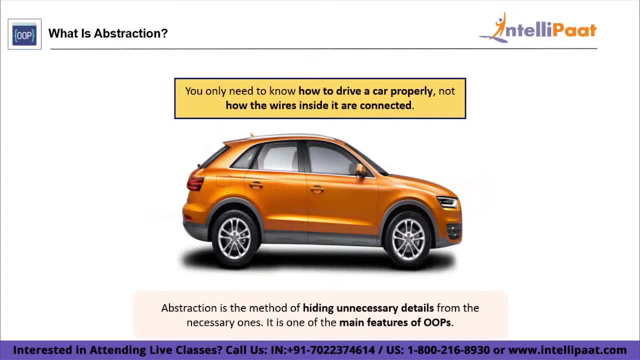 For example, consider a car. If you want to drive a car, you don't need to know how the wires in the car are connected right, And that is unnecessary detail for you. You just need to know how to drive a car. 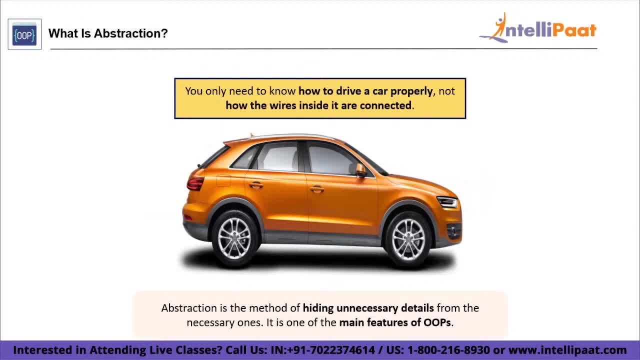 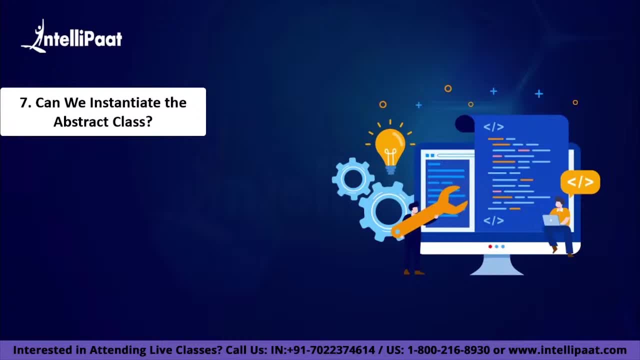 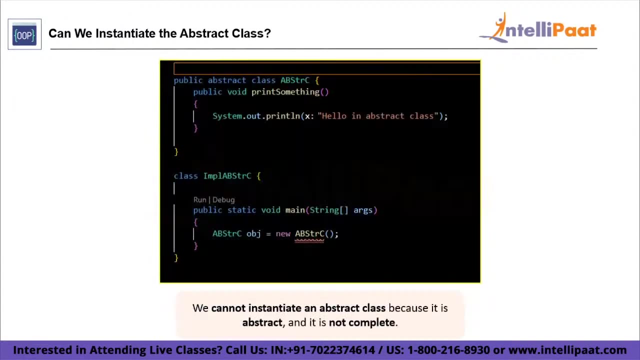 And that is the exact process abstraction gives us. Now, moving ahead, we'll explore a few tricky questions. The question I'm going to begin with is: can we instantiate the abstract class? The answer to this question is no, We cannot instantiate. We cannot instantiate an abstract class in Java because it is abstract and it is not complete. 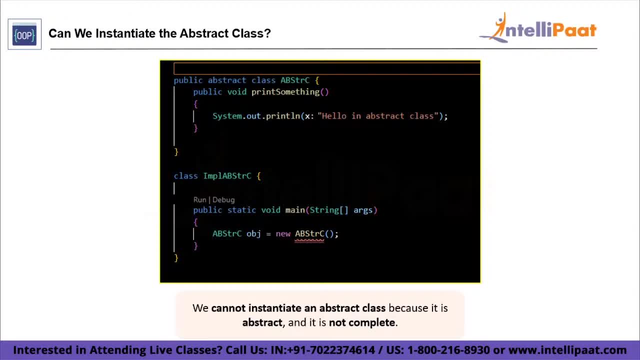 Let me give you proof of this argument. Here is a Java program where we are trying to instantiate the abstract class, And this is the result we get after performing this operation: That is, cannot instantiate the type function name. So basically, what this is telling is: you cannot instantiate the method from abstract class. 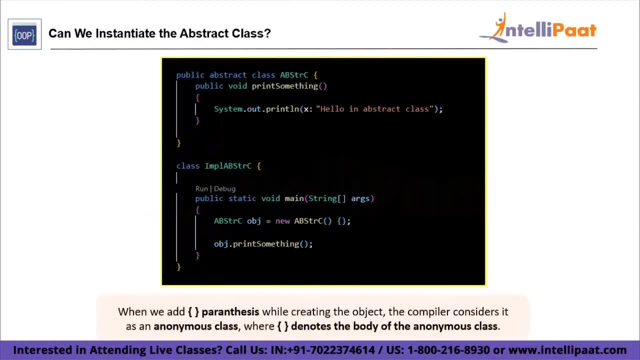 I have one more program here. What do you think? Will it be able to instantiate the abstract class? Well, let me tell you this program is not of instantiation Here. in this second example, the object of abstract class is not created, but the instance of anonymous subclass of abstract class has been created. 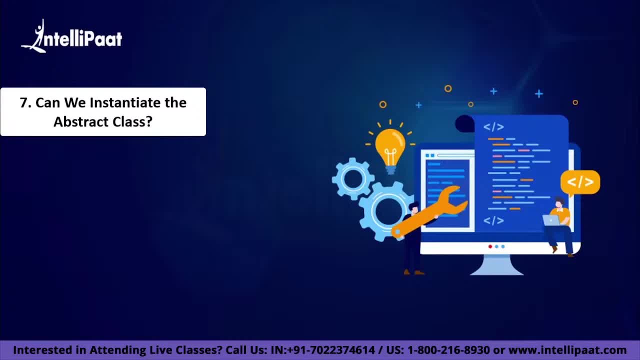 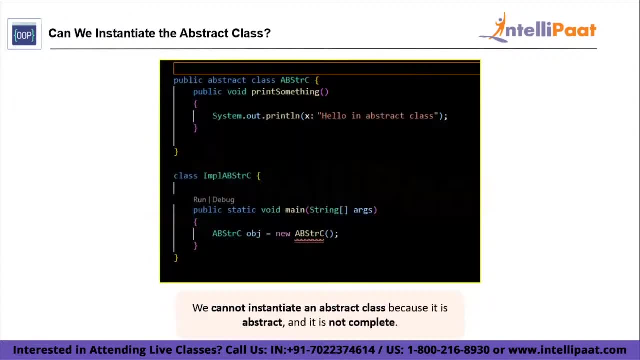 a few tricky questions. The question I'm going to begin with is: can we instantiate the abstract class? is no, We cannot instantiate an abstract class in java because it is abstract and it is not complete. Let me give you proof of this argument. Here is a java program where we are trying. 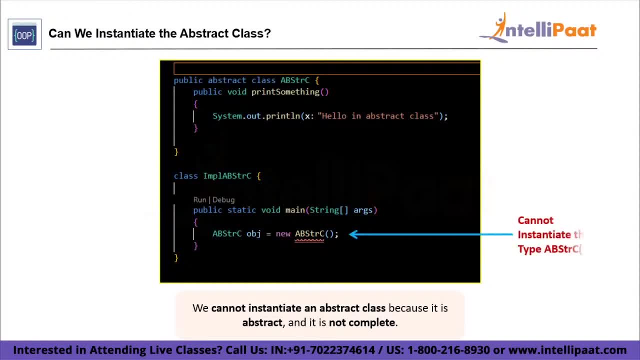 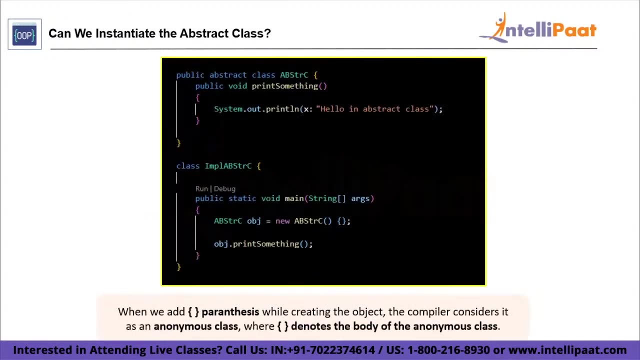 to instantiate the abstract class, and this is the result we get after performing this operation: That is, cannot instantiate the type function name. So, basically, what this is telling is: you cannot instantiate the method from abstract class. I have one more program here. What do you think? Will it be able to instantiate the abstract class? Well, let me. 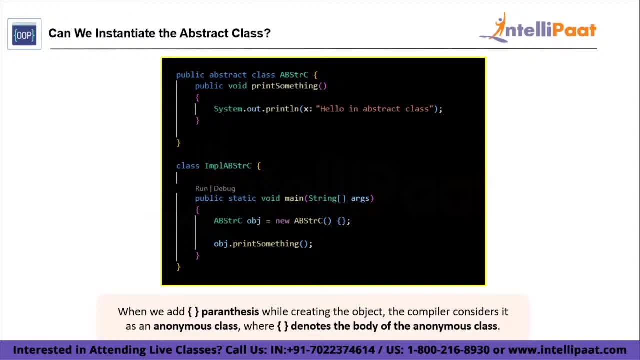 tell you this program is not of instantiation Here. in this second example, the object of abstract class is not created, but the instance of anonymous subclass of abstract class has been created. And then we are invoking the method print something on the abstract class reference pointing to subclass object obj, When you have added curly parenthesis, while. 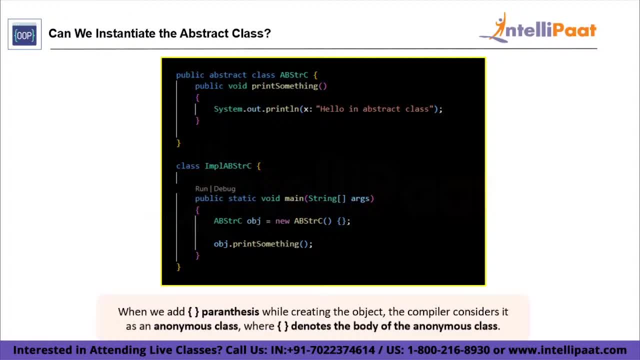 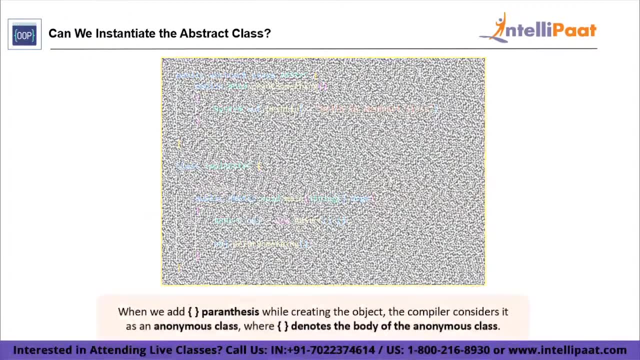 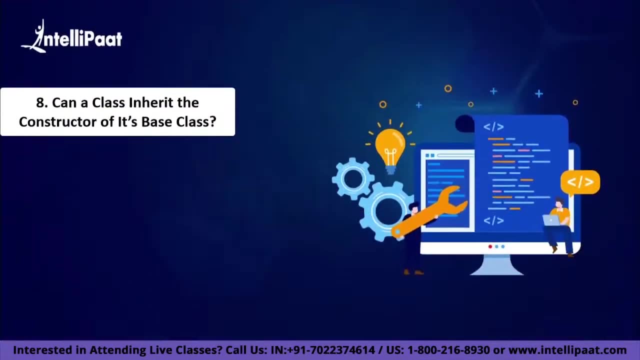 creating the object in second class, The compiler takes it as an anonymous class, where curly parenthesis denotes the body of anonymous class. So even though we implement abstract class method here, this won't be the example of inheritance. Now the eighth question on our list is: is it possible for a class 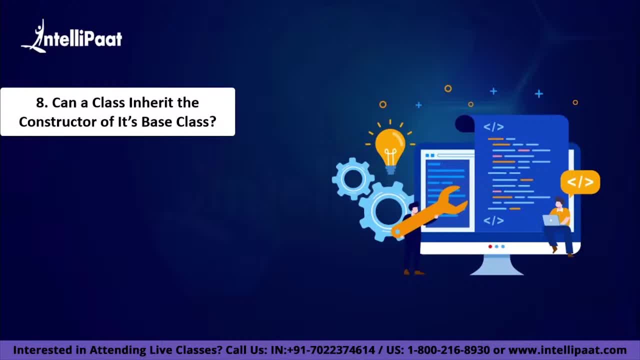 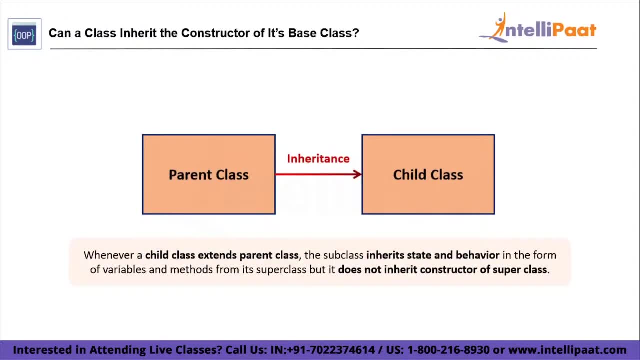 to inherit the constructor of its base class? The answer to this question is no. Whenever a child class extends a parent class, the subclass inherits state and behavior in the form of variables and methods, But it does not inherit constructor of superclass, because constructors are special and have 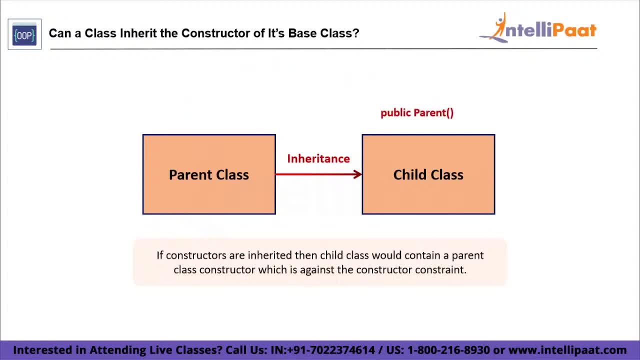 the same name as class name. So if constructor were inherited in child class, then child class would contain a parent class constructor, which is against the constraint that constructor should have same name as class name. And this is not happening if we are invoking the constructor of parent class inside the base class, right? So that is why a class cannot inherit the 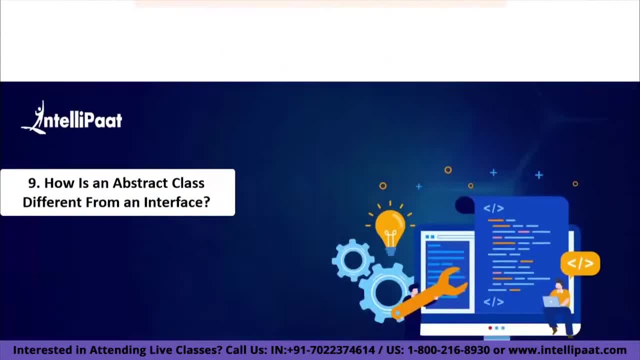 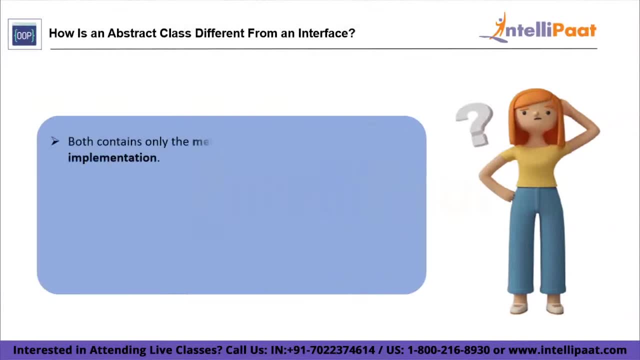 constructor of its base class. Now, next question we have on our list is: how is an abstract class different from an interface? Interface and abstract classes: both are special types of classes that contain only the method declaration and not their implementation, But the interface is entirely different from. 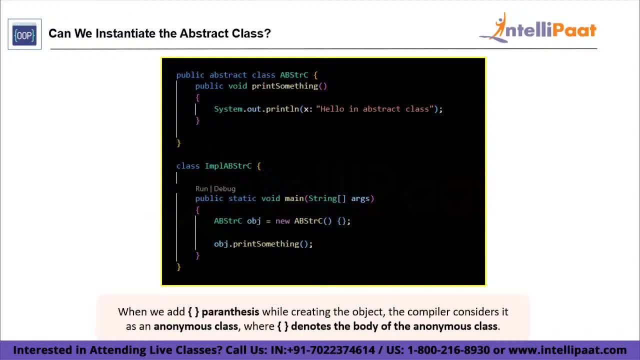 And then we are invoking the method print something on the abstract class reference pointing to subclass object OBJ. When you have added curly parenthesis while creating the object in second class, the compiler takes it as an anonymous class, where curly parenthesis denotes the body of anonymous class. 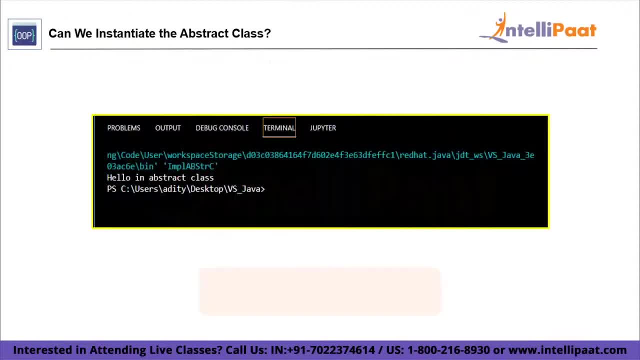 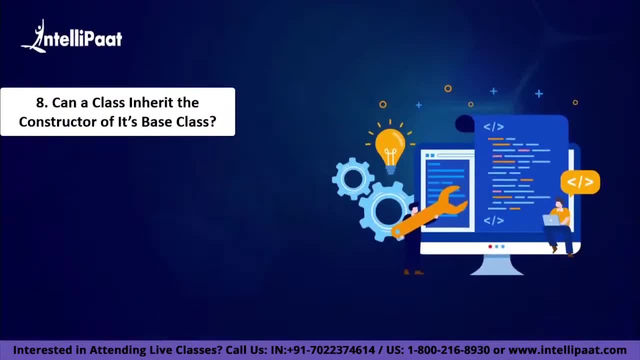 So, even though we implement abstract class method here, this won't be the example of inheritance. Now the eighth question on our list is: is it possible for a class to inherit the constructor of its base class? The answer to this question is no. 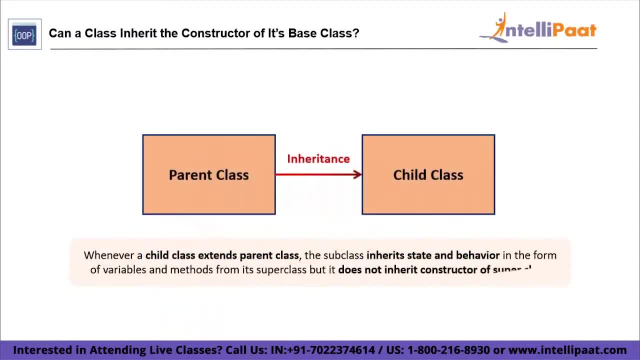 Whenever a child class extends a parent class, the subclass inherits state and behavior in the form of variables and methods from its superclass, But it does not inherit constructor of superclass, Because constructors are special and have the same name as class name. So if constructor were inherited in child class, 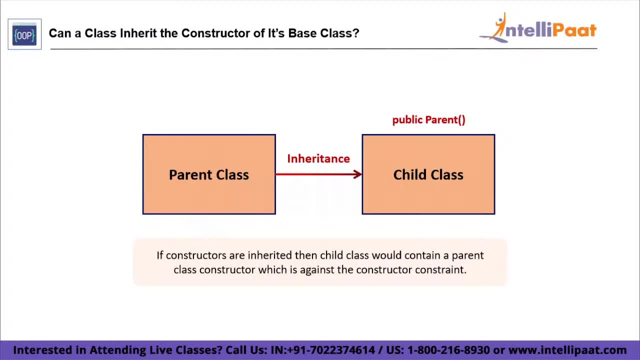 then child class would contain a parent class constructor, which is against the constraint that constructor should have same name as class name. And this is not happening if we are invoking the constructor of parent class inside the base class right. So that is why a class cannot inherit constructor of its base class. 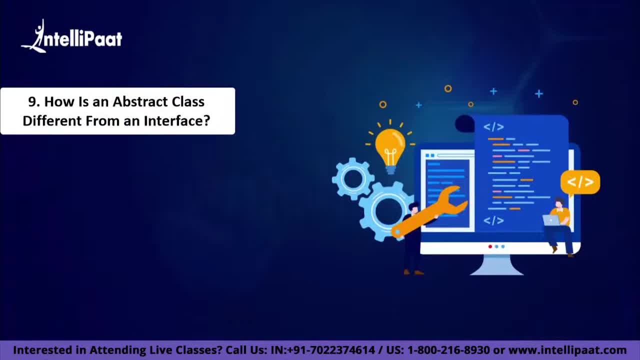 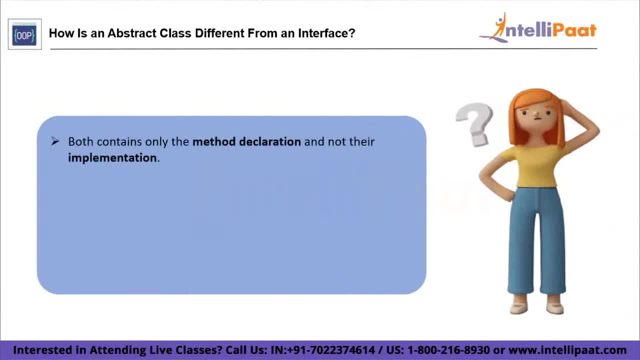 Now next question We have on our list is: how is an abstract class different from an interface, Interface and abstract classes? both are special types of classes that contain only the method declaration and not their implementation. But the interface is entirely different from an abstract class. 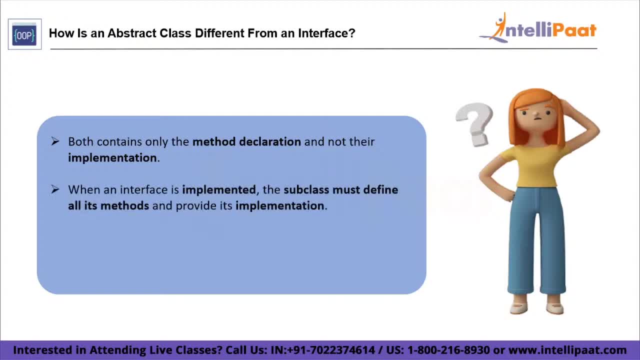 The main difference between the two is that when an interface is implemented, the subclass must define all its methods and provide its implementation, Whereas when an abstract class is inherited, the subclass does not need to provide any definition of its abstract method until and unless the subclass is using it. 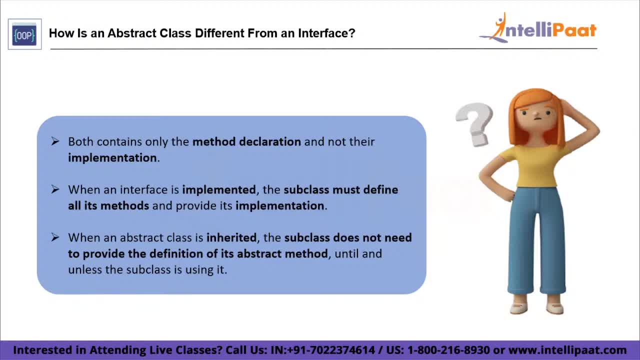 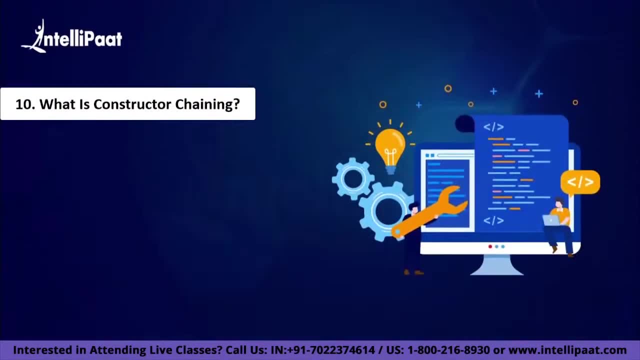 Also, an abstract class can contain abstract methods as well as non-abstract methods, which is not the case with interfaces. That brings us to the 10th question on our list. Explain constructor chaining. In OOPS, constructor chaining is a sequence of invoking constructors. 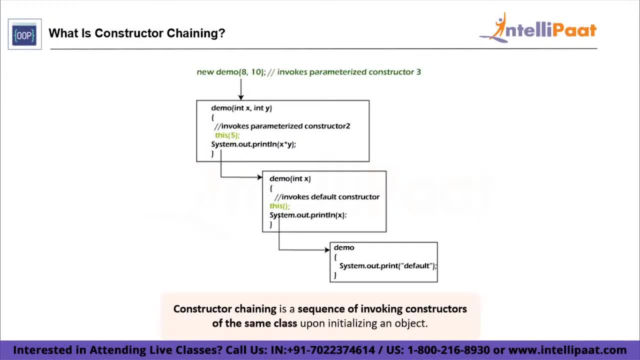 of same class upon initializing an object. It is used when we want to invoke a number of constructors, one after another, using only an instance. For example, you can look at this demo function here: The first call is new demo 8 comma 10.. 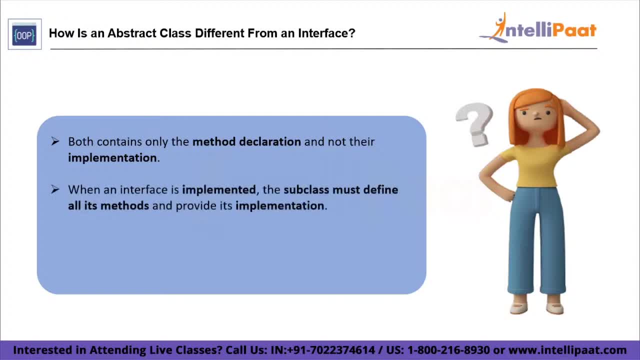 an abstract class. The main difference between the two is that when an interface is implemented, the subclass must define all its methods and provide its implementation, Whereas when an abstract class is inherited, the subclass does not need to provide any definition of its abstract method until and unless the subclass is using it. Also, an abstract class can contain: 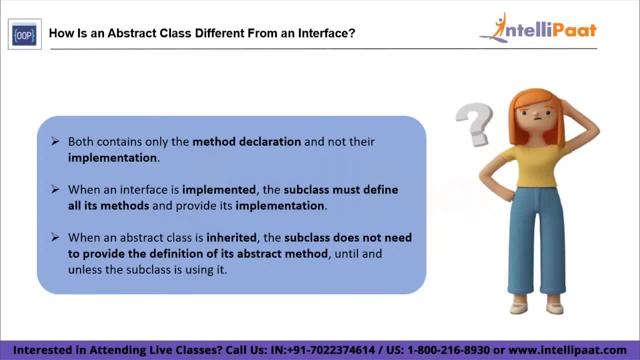 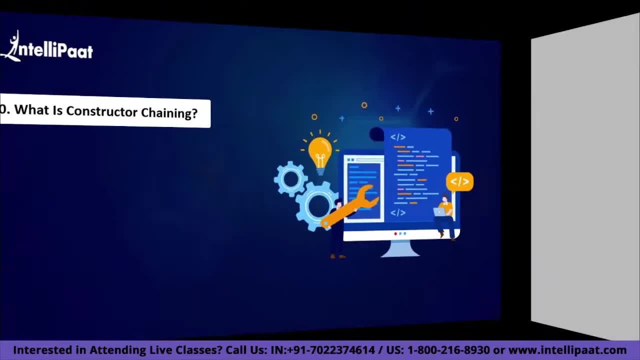 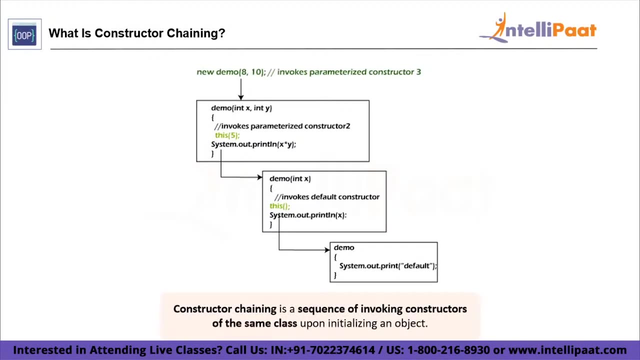 abstract methods as well as non-abstract methods, which is not the case with interfaces. That brings us to the 10th question on our list: Explain constructor chaining. In OOPS, constructor chaining is a sequence of invoking constructors of same class upon initializing an object. It is used when we 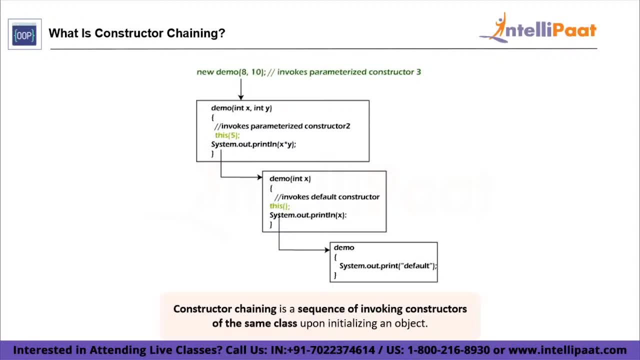 want to invoke a number of constructors, one after another, using only an instance. For example, you can look at this demo function here: The first call is new demo 8, comma 10, and again inside that block we are mentioning the this function which is giving to the demo. 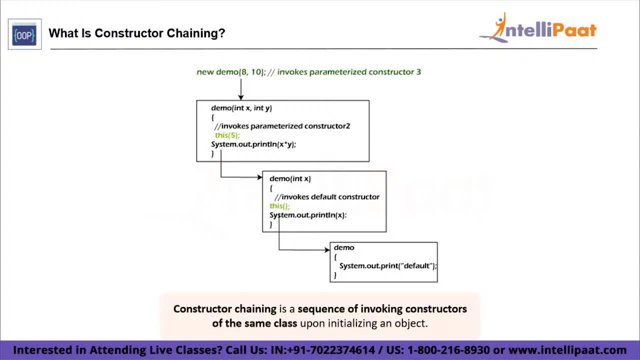 function call, again with only one parameter, and similarly, inside that function block, again using this call, with no parameter. What I am trying to say here is, in other words, if a class has more than one constructor, then it should be able to invoke a number of constructors. 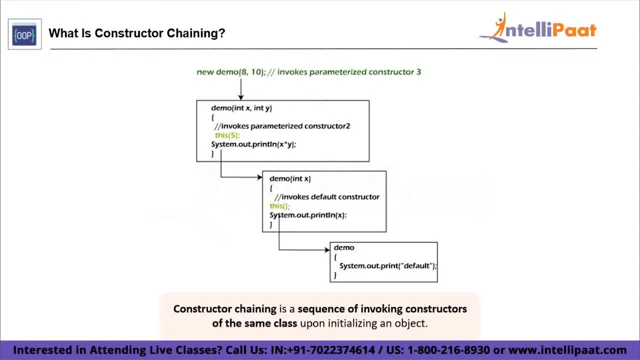 more than one constructor and one of them tries to invoke another constructor. This process of chaining is called as constructor chaining. It is known as constructor delegation in C++ programming language. Now let's move to the 11th question. What is a singleton class and how is it different? 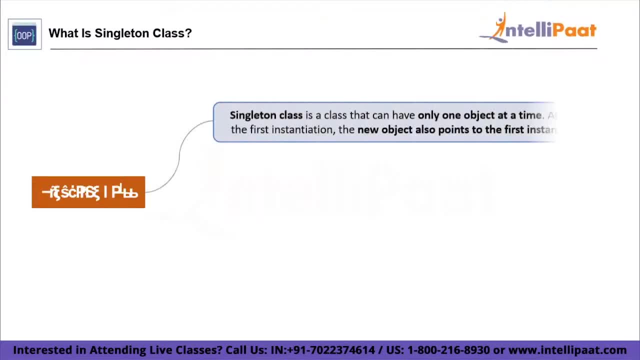 from static class. In object oriented programming, a singleton class is a class that can have only one object. After the first time, if we try to instantiate the singleton class, the new variable also points to a class. This class is called a class When we try to instantiate. 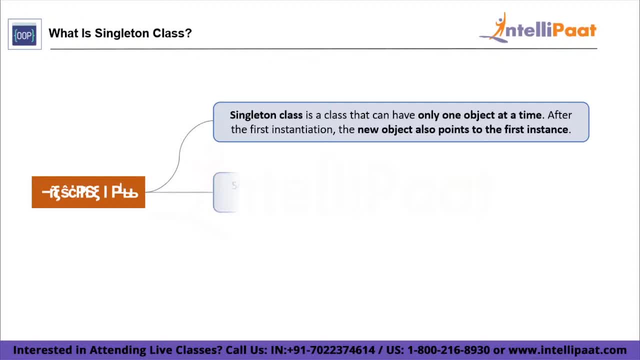 the class, the new variable also points to a class. When we try to instantiate the class, the new variable also points to the first instance created. So whatever modification we do to any variable inside the class through instance affects the variable of the single instance created and is visible if we access that variable through any variable that we 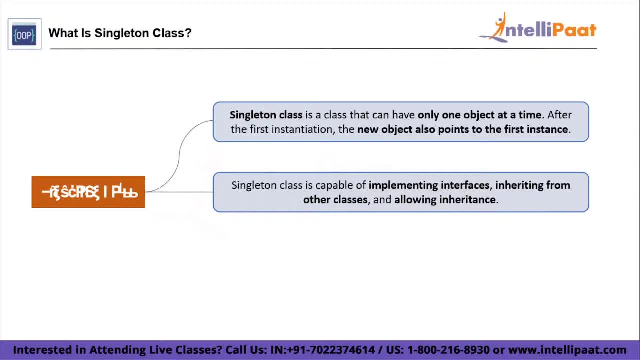 have for an object. This singleton class is capable of implementing interfaces inheriting from other classes and allowing inheritance. A static class, on the other hand, cannot inherit its instance members. As a result, Singleton classes are considered more accurate and can considered more adaptable than static classes. 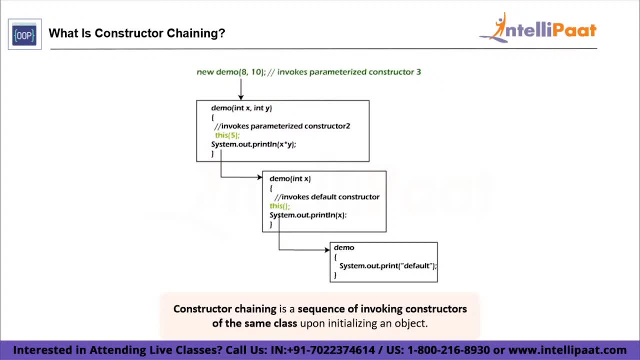 And again inside that block. we are mentioning that this function, which is giving to the demo function call, again with only one parameter, And similarly inside that function block, again using this call, with no parameter. What I'm trying to say here is, in other words, if a class has more than one, 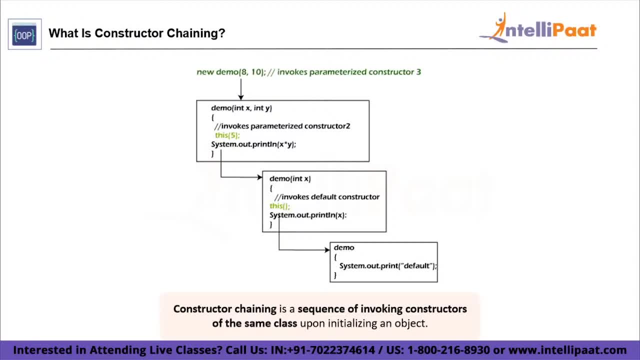 constructor and one of them tries to invoke another constructor. this process of chaining is called as constructor chaining. It is known as constructor delegation in C++ programming language. Now let's move to the 11th question. What is a singleton class and how is it different from static class? 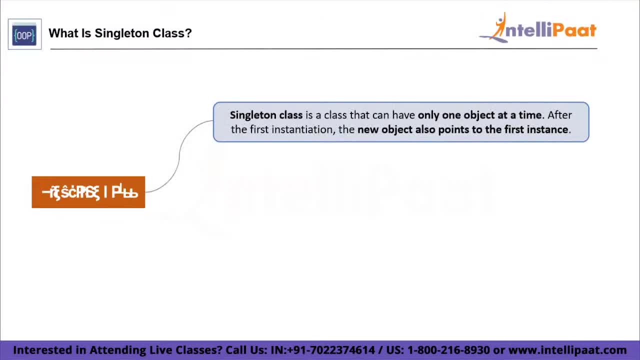 In object oriented programming a singleton class is a class that can have only one object After the first time. if we try to instantiate the singleton class, the new variable also points to the first instance created. So whatever modification we do to any variable inside the class through instance affects the variable. 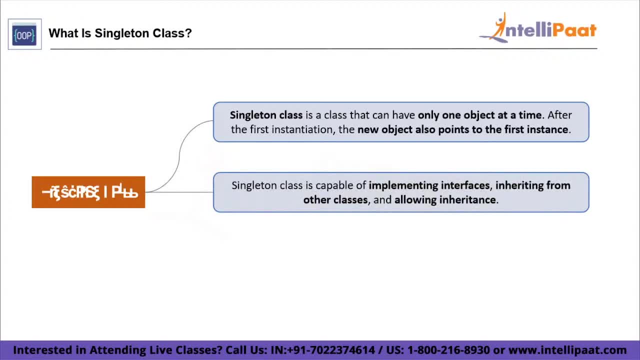 of the single instance created and is visible if we access that variable through any variable that we have for an object. This singleton class is capable of implementing interfaces inheriting from other classes and allowing inheritance. A static class, on the other hand, cannot inherit its instance members. 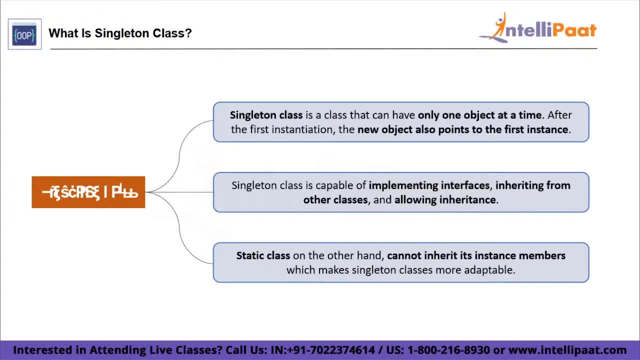 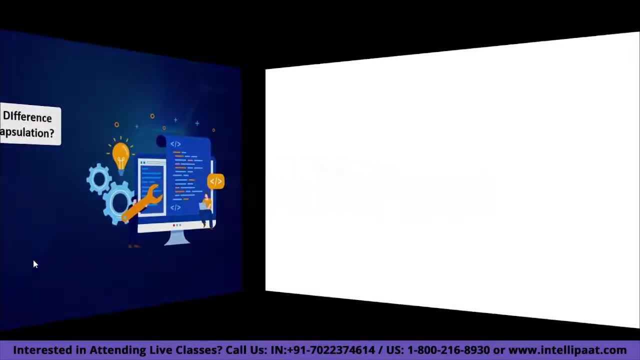 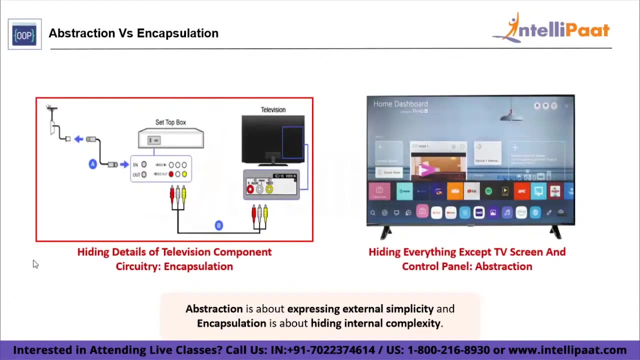 As a result, singleton classes are considered more adaptable than static classes. Next up is: what is the fundamental difference between abstraction and encapsulation? This is a difficult question. Most candidates attempt to explain and define both terms, However, when they stress about differences. 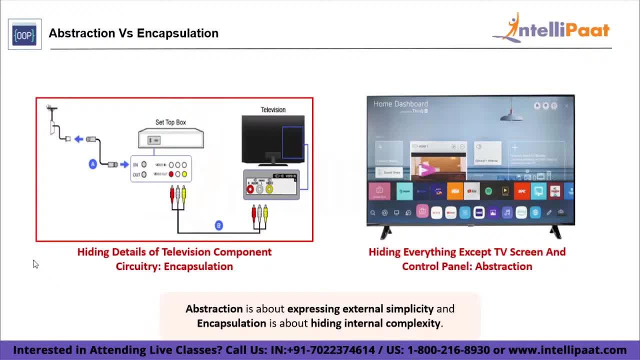 they become confused and do not respond to this question. because abstraction and encapsulation- both are employed to hide the stuff. right, But here is the difference: Abstraction is about expressing external simplicity and encapsulation is about hiding internal complexity. Let's say we want. 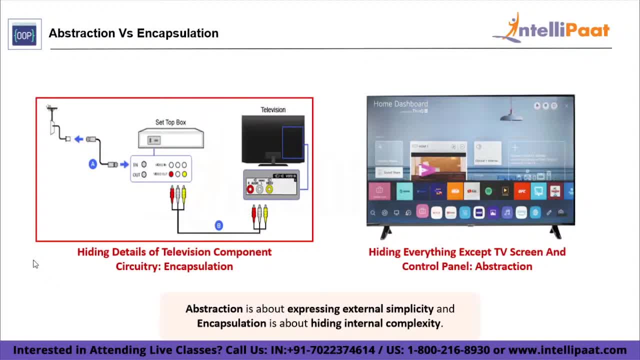 a user to interact with an object called television by using either of these methods. Using encapsulation, you would hide all the wiring and component circuitry because no one needs to understand how all the engineering works in order to watch TV. Here we are actually hiding the internal complexity of TV, right. 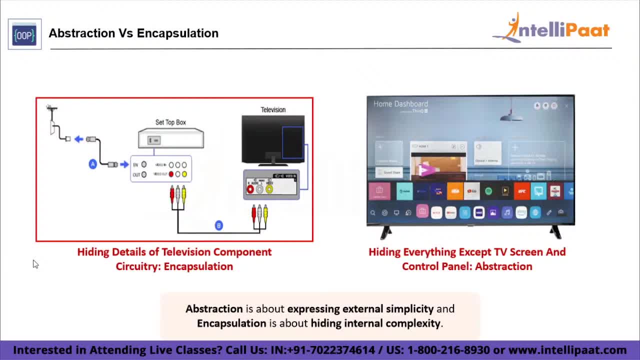 Whereas if we employ abstraction, you would hide everything but the TV screen and the clicker interface, So you could see the picture and use the control. This is all about expressing important information and hiding unimportant details. So this is the basic difference between abstraction and encapsulation. 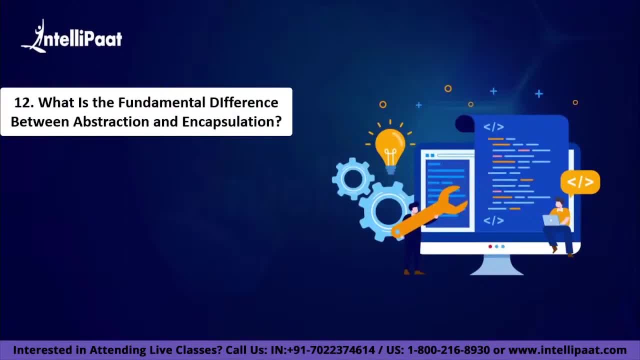 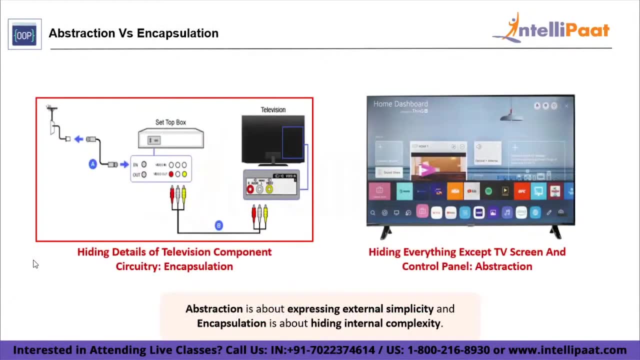 Next up is: what is the fundamental difference between abstraction and encapsulation? This is a difficult question. Most candidates attempt to explain and define both terms. However, when they are stressed about differences, they become confused and do not respond to this question. because abstraction and encapsulation- both are employed to hide the stuff right. 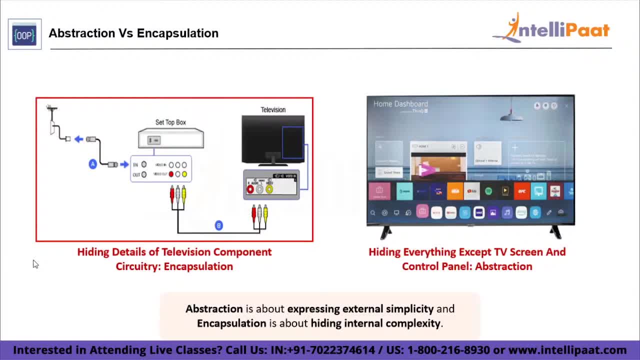 But here is the difference: Abstraction is about expressing external simplicity and encapsulation is about hiding internal complexity. Let's say we want a user to interact with an object called television by using either of these methods. Using encapsulation, you would hide all the wiring and component circuitry because no one needs to understand how all the engineering. 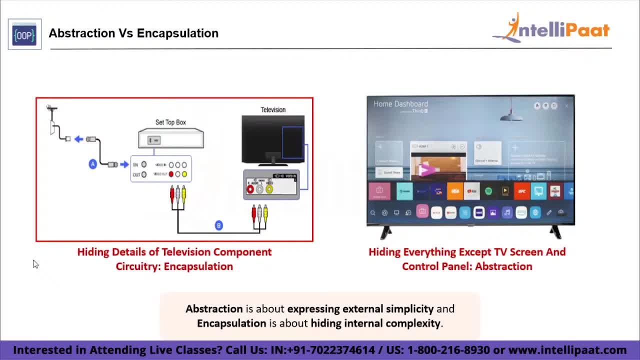 works in order to watch TV. Here we are actually hiding the internal complexity of TV right, Whereas if we employ abstraction, you would hide everything but the TV screen and the clicker interface so you could see the picture and use the control. This is all about expressing important information and hiding unimportant. 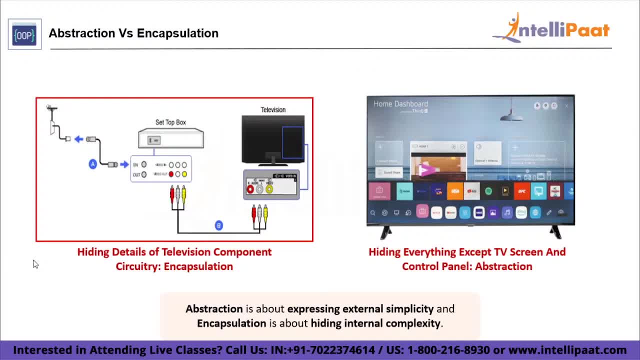 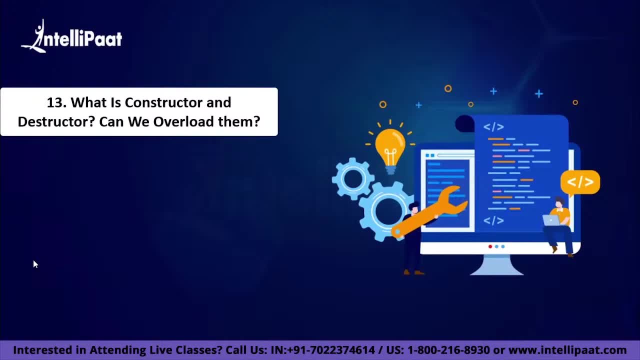 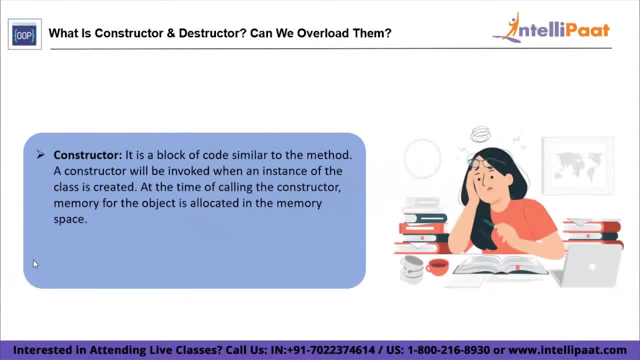 details. So this is the basic difference between abstraction and encapsulation. This brings us to the 13th question on our list: What is constructor and destructor, and can we overload them? A constructor is a block of code similar to the method It is called when an instance of the class is created At the time of calling. 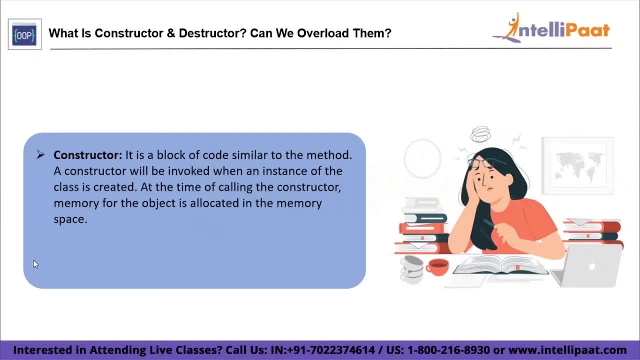 the constructor, memory for the object is allocated in the memory space. It is a space spatial type of method which is used to initialize the objects. Destructor is an instance member that is called whenever an object is about to be destroyed. In other words, a destructor is the last function that is called before an object is destroyed. 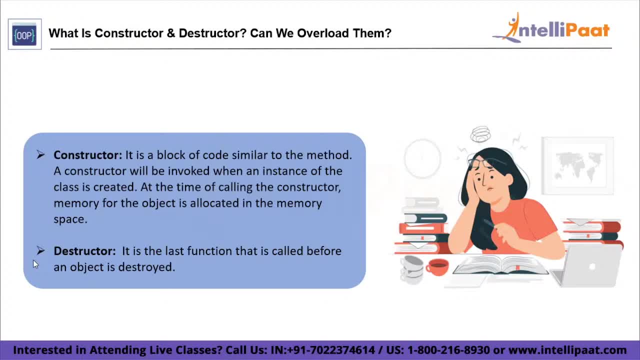 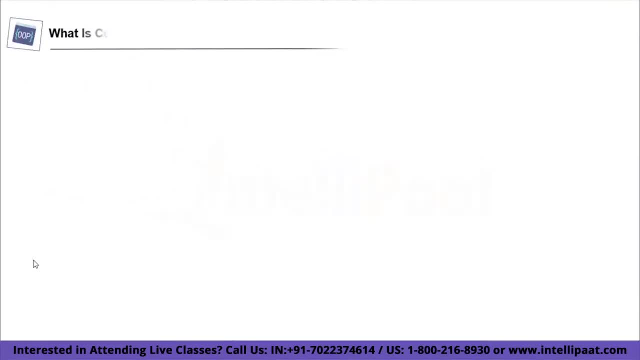 Both this constructor and destructor of base class cannot be overloaded in its child class 14.. What is Composition? The composition is a way to design or implement. a has a relationship. Composition trains the user and havoc, rather than an abstract macaroni or original competition. Rainer T Weber Composition. 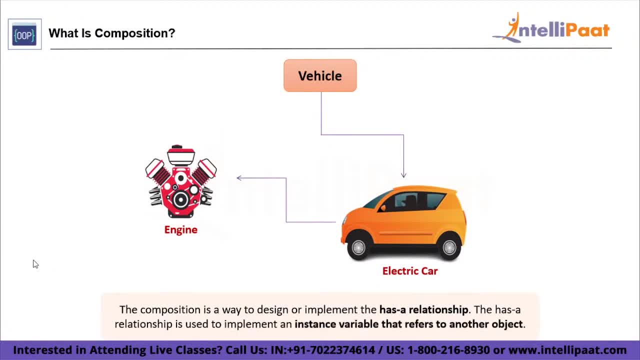 Composition and inheritance. both are design techniques. The inheritance is used to implement, is a relationship, whereas the has a relationship is used to ensure code reusability. in our program, In composition, we use an instance variable that refers to another object. The composition relationship of two objects is possible when one object contains another. 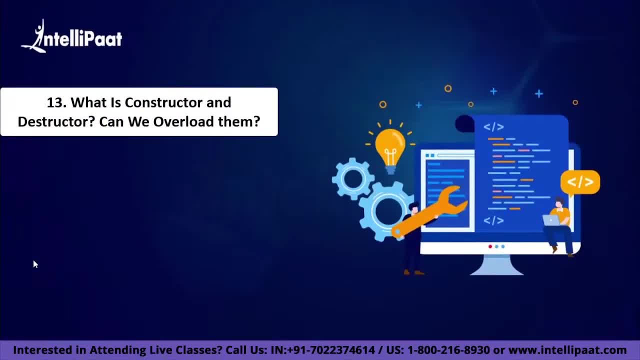 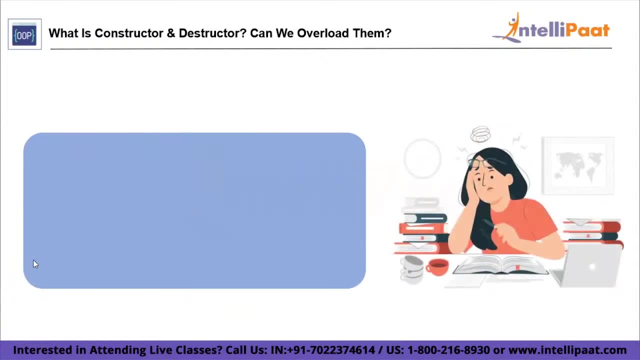 This brings us to the 13th question on our list: What is constructor and destructor, and can we overload them? A constructor is a block of code similar to the method. It is called when an instance of the class is created At the time of calling the constructor. 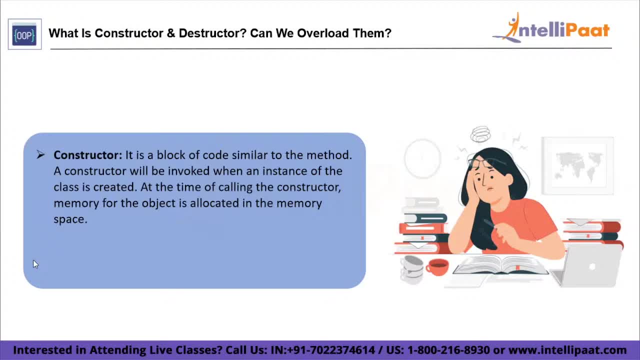 memory for the object is allocated in the memory space. It is a special type of method which is used to initialize an object, whereas destructor is an instance member that is called whenever an object is about to be destroyed. In other words, a destructor is the last. 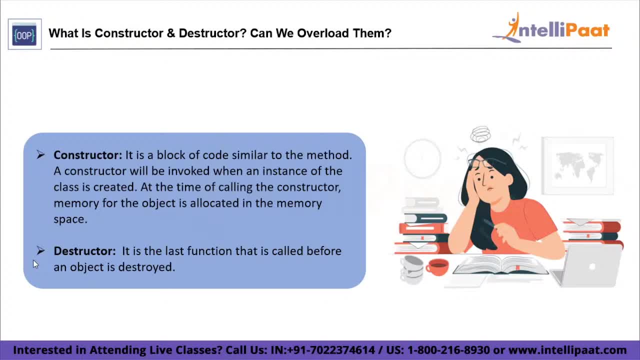 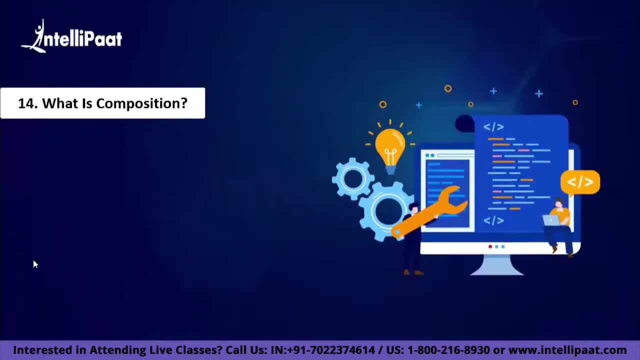 function that is called before object is destroyed. Both this constructor and destructor of base class cannot be overloaded in its child class. Now let's move to the question number 14.. What is composition? The composition is a way to design or implement a hazard relationship. 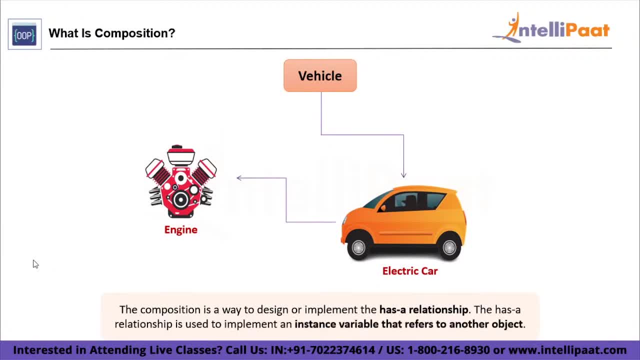 Composition and inheritance. both are design techniques. The inheritance is used to implement, is a relationship, whereas the hazard relationship is used to ensure code reusability. in our program, In composition we use an instance variable that refers to another object. The composition relationship of two objects is possible when one object 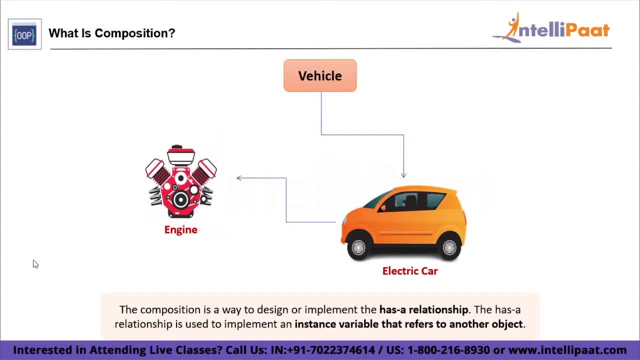 contains another object and that object is fully dependent on it. For example, consider this example- The electric car contains an engine and every electric car is a vehicle. So in between vehicle and electric car we have is a relationship because electric car is a vehicle and electric car has an engine. 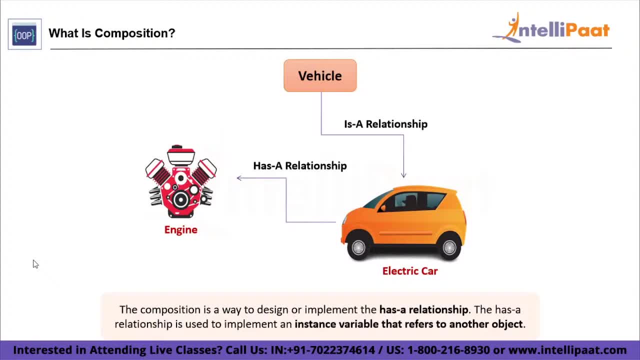 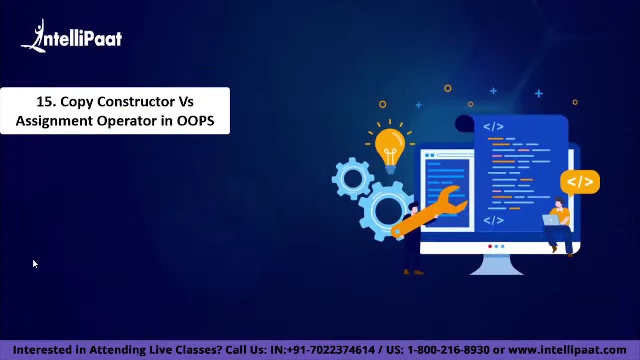 So that's why that is a composition. I hope this is pretty clear to all of you guys now. Now let's move to the next question on our list. What are the differences between copy constructor and assignment operator, The copy constructor and the assignment? 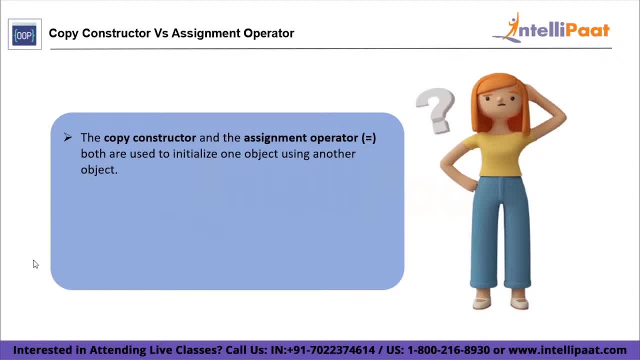 operator. both are used to initialize one object using another object. The main difference between the two is that the copy constructor allocates separate memory to both objects, that is, existing object and newly created object, while the assignment operator does not allocate new memory for the newly. 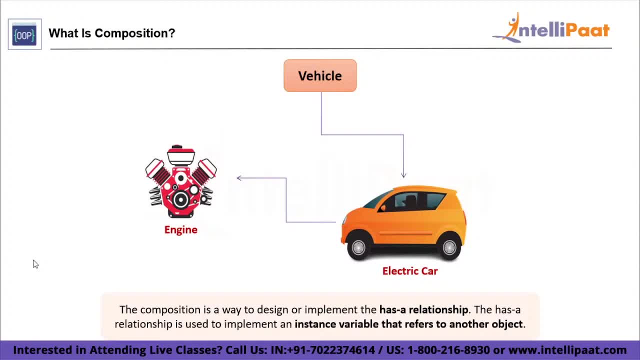 object and that object is fully dependent on it. For example, consider this example- The electric car contains an engine and every electric car is a vehicle. So in between vehicle and electric car we have is a relationship because electric car is a vehicle and electric car has an engine. 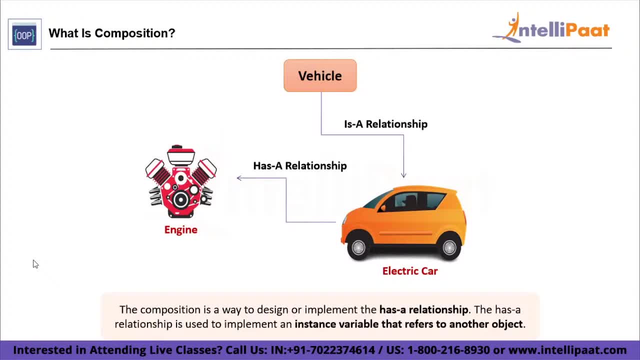 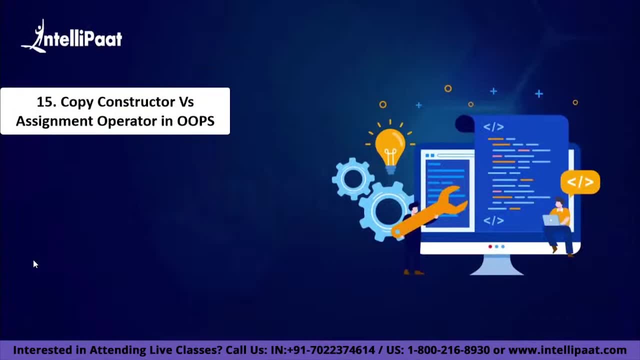 So that's why that is a composition. I hope this is pretty clear to all of you guys now. Now let's move to the next question on our list. What are the differences between copy constructor and assignment operator? The copy constructor and the assignment operator. Both are used to initialize one object using another object. The main difference between the two is that the copy constructor allocates separate memory to both objects, That is, existing object and newly created object, while the assignment operator does not allocate new memory for the newly created object. 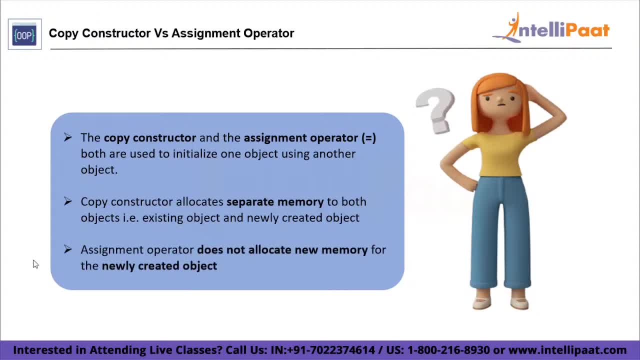 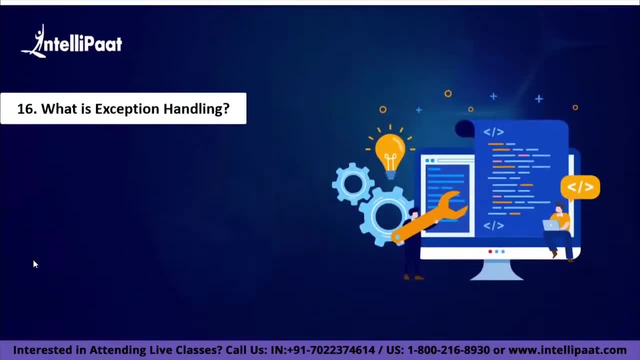 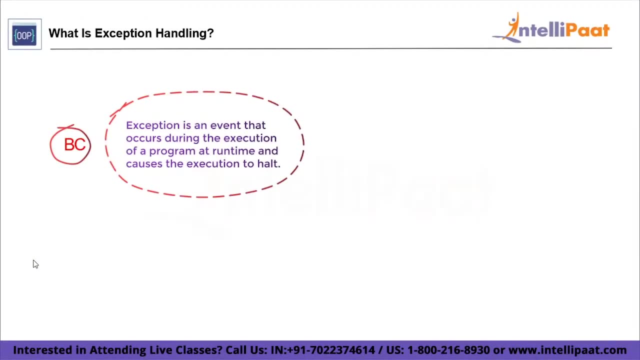 It uses the reference variable that points to the previous memory block where an old object is located. I hope this difference is clear to all of you guys. Now let's move to the 16th question on our list: What is Exception Handling? First of all, let's understand what an exception is. 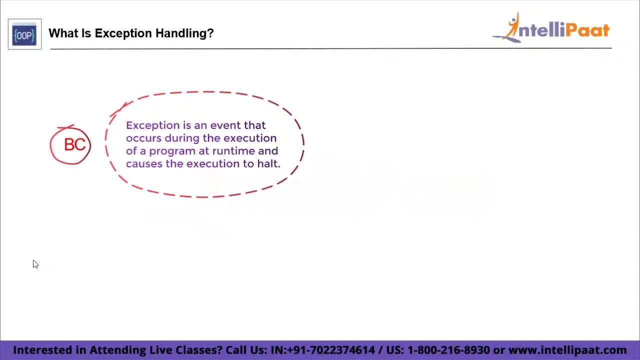 Exception is nothing but a special event that occurs during the execution of a program at runtime and causes the execution to halt. The reason for the exception is primarily due to a position in a program where a user wishes to do something that the program does not support. 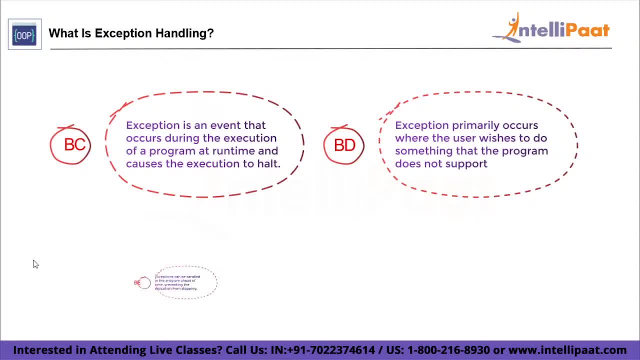 For example, undesirable input addition. Nobody wants their software to malfunction or crash. Exception is the most common example of an exception. Exception is the most common example of an exception, The most common cause of software failure. Exceptions can be handled in the program ahead of time, preventing the execution from stopping. 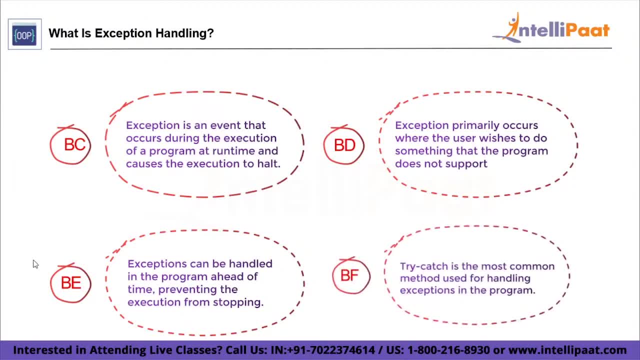 This is known as Exception Handling. So Exception Handling is a mechanism for identifying the undesirable states that the program can reach and specifying the desirable outcomes for each state. Try-catch is the most common method used for handling exceptions in the programming languages. Now let's move to the 17th question. 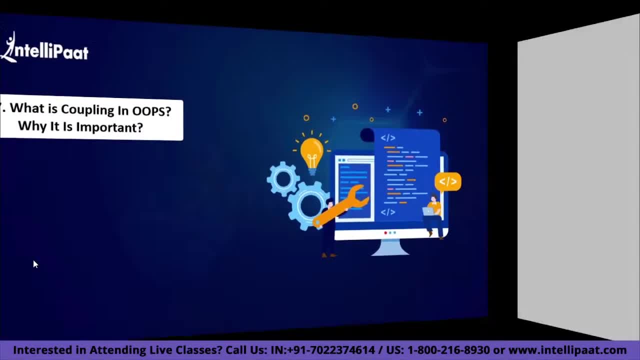 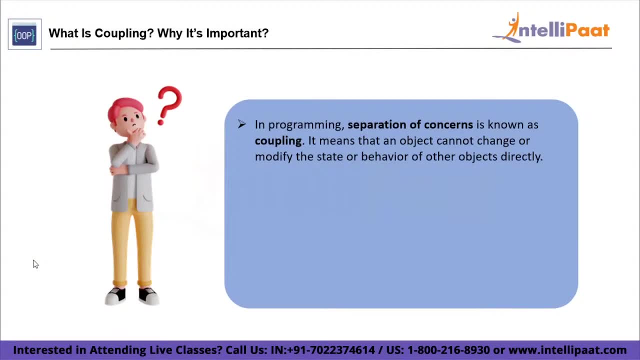 That is what is coupling in OOP and why it is helpful In programming. separation of concerns is known as coupling. It means that an object cannot change or modify the state or behavior of other objects directly. It describes how closely two objects are linked. 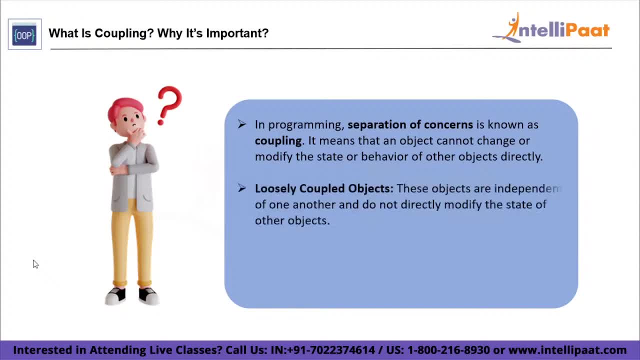 Loose coupling and tight coupling are the two types of coupling. Objects that are loosely coupled are those that are independent of one another and do not directly modify the state of other objects. Loose coupling makes the code more adaptable. Change the state of other objects. 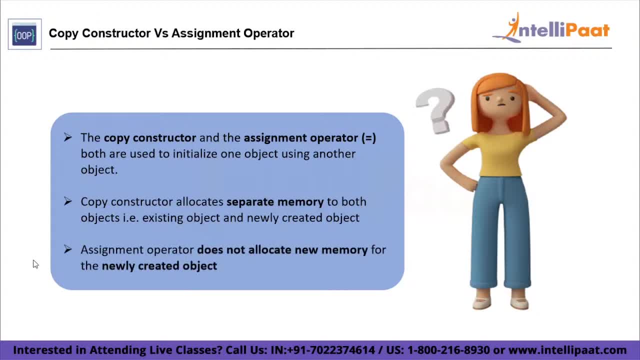 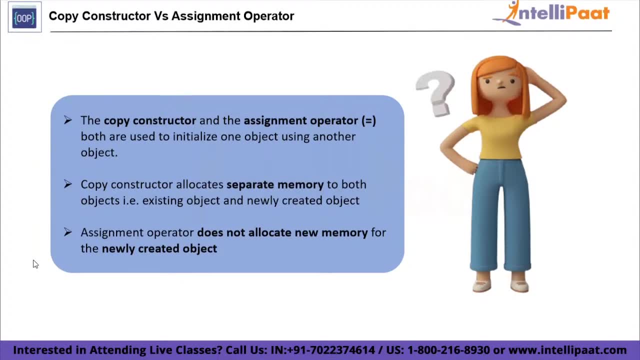 created object. It uses the reference variable that points to the previous memory block where an old object is located. I hope this difference is clear to all of you guys. Now let's move to the 16th question on our list: What is exception handling? First of all, let's understand. 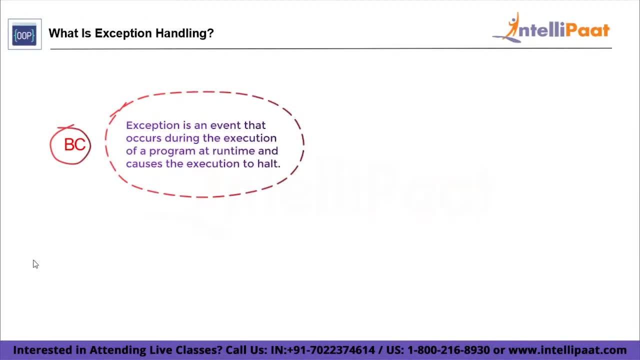 what an exception is. Exception is nothing but a special event that occurs during the execution of program at runtime and causes the execution to halt. The reason for the exception is primarily due to a position in a program where a user wishes to do something that the program does not support. 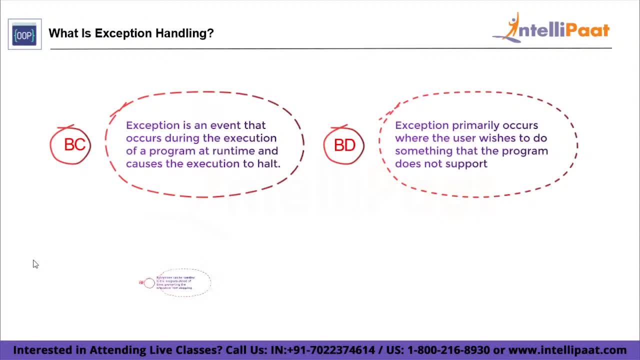 For example, undesirable input addition. Nobody wants their software to malfunction or crash. Exceptions are the most common cause of software failure. Exceptions can be handled in the program ahead of time, preventing the execution from stopping. This is known as exception handling. So exception handling is a mechanism for identifying the undesirable states. 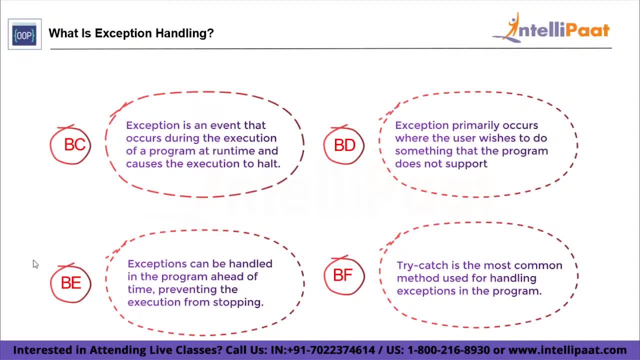 that the program can reach and specifying the desirable outcomes for each state. Try-catch is the most common method used for handling exceptions in the programming languages. Now let's move to the 17th question, That is, what is coupling in OOP and why it is helpful. 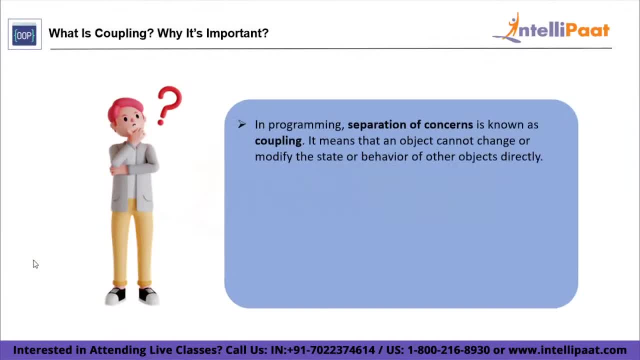 In programming, separation of concerns is known as coupling. It means that an object cannot change or modify the state or behavior of other objects directly. It describes how closely two objects are linked. Loose coupling and tight coupling are the two types of coupling. Objects that are loosely coupled are those that are independent of one another. 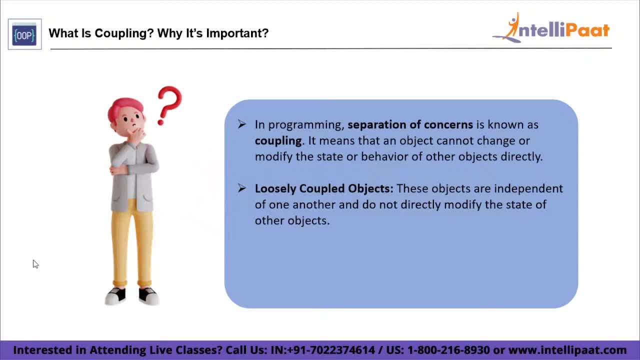 and do not directly modify the state of other objects. Loose coupling makes the code more adaptable, changeable and user friendly, Whereas objects that depend on other objects and can modify their states are called as tightly coupled. It creates conditions where modifying the code of one object also requires changing. 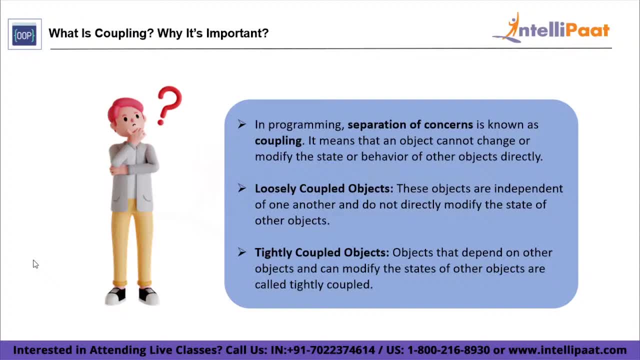 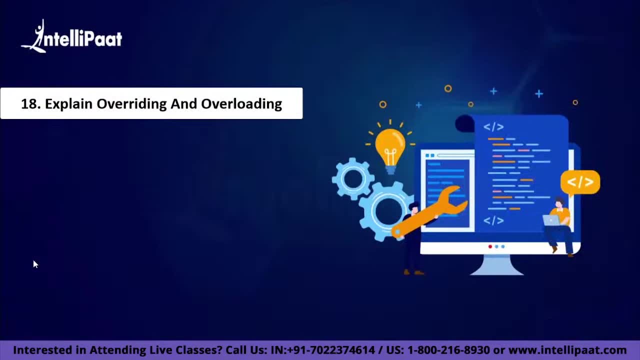 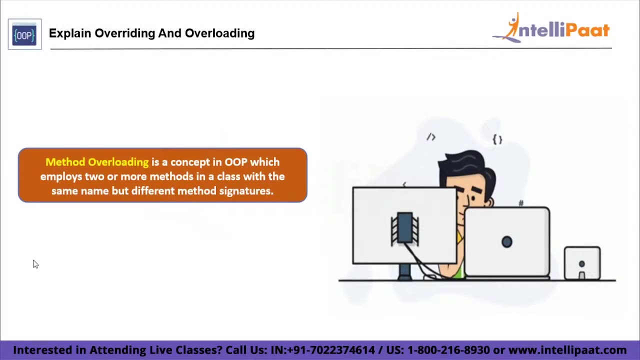 the code of other objects. The reuse of code is difficult in this case. That is why using loose coupling is always a good habit. Now let's move to the 18th question on our list: Explain overloading and overriding. Overloading is a concept in object oriented programming when two or more methods in a class with same name but 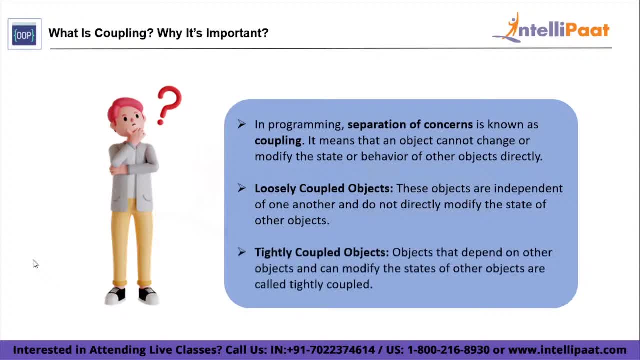 Changeable and user-friendly, Whereas objects that depend on other objects and can modify their states are called as tightly coupled. It creates conditions where modifying the code of one object also requires changing the code of other objects. The reuse of code is difficult in this case. 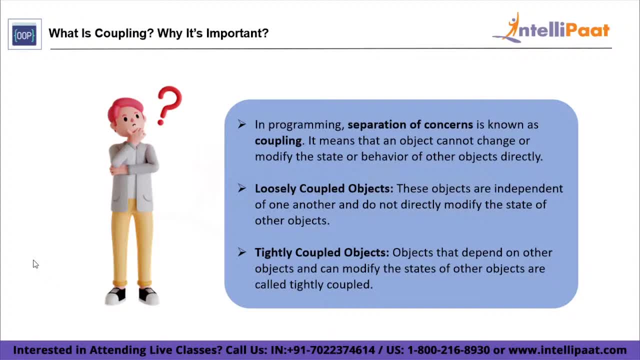 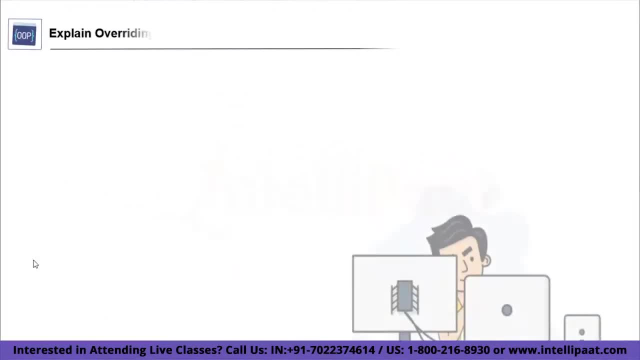 That is why using loose coupling is always a good habit. Now let's move to the 18th question on our list, Explain overloading and overriding. Overloading is a concept in OOP. It is a method of integrated programming when two or more methods in a class with same name. 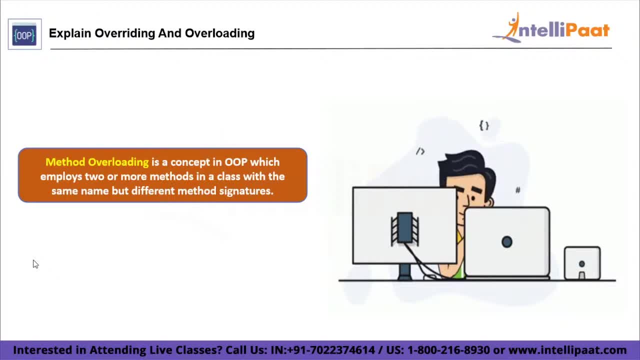 but different signature exist. It is also known as compile-time polymorphism. If a method with same method signature is presented in both child and parent class, then it is known as overriding. The methods must have the same number of parameters and the same type of parameter. 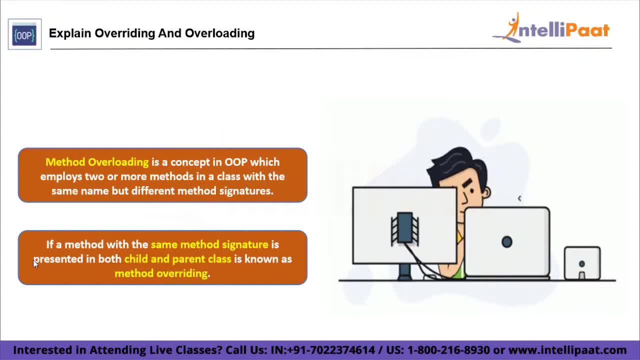 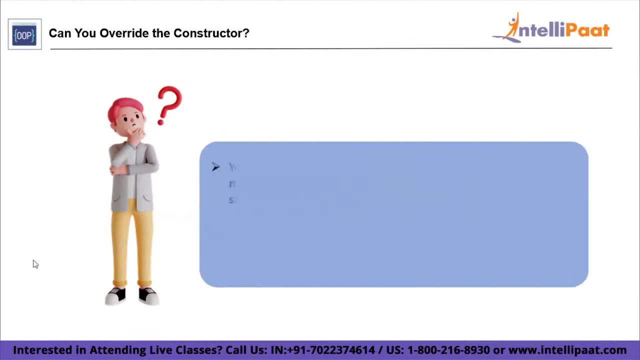 This is also known as runtime polymorphism as well. Now next question we have on our list is: can you override the constructor? Well, You cannot override the constructor, because it looks like a method, but it is not. It lacks a return type and shares the same name as a class. 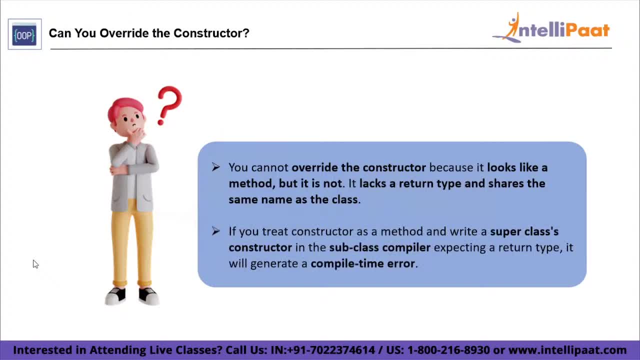 If you treat it as a method and write a superclass as constructor in the subclass compiler, expecting a return type will generate a compile-time error, So you cannot actually override the constructor. Now. finally, the last question on our list is if you have a class containing a static. 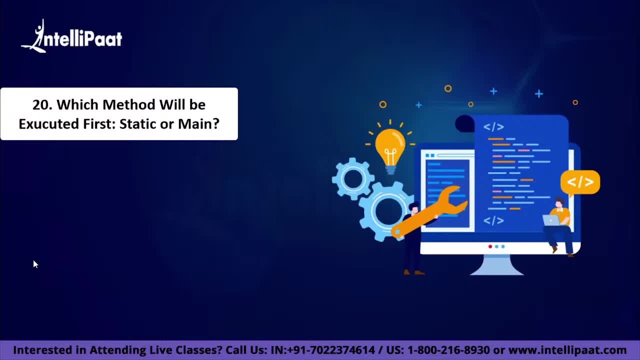 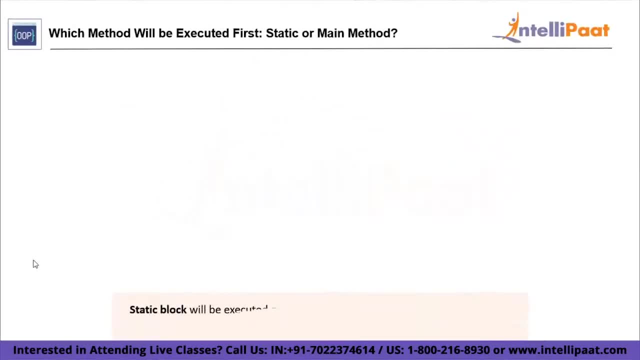 method and main method with the print statement. Which print statement will be executed? Now? this is a tricky question, But the answer to this is pretty straight forward. Many languages execute static block on priority basis. What it simply means is static block will be executed even before the compiler or interpreter. 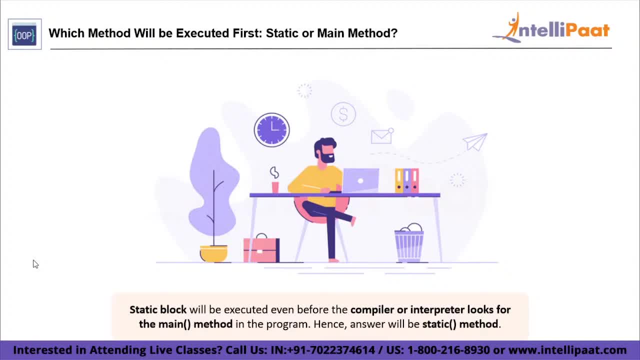 looks for main method in program. Once the static method is executed, the main method will be compiled. Hence the answer to this question will be: print statement in the static method will be executed first. That's all we have for this session. Thank you so much for watching. 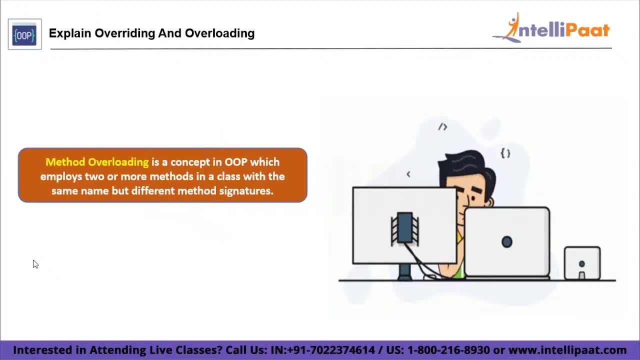 different signature exist. It is also known as compile time polymorphism. If a method with same method signature is presented in both child and parent class, then it is known as overriding. The methods must have the same number of parameters and the same type of parameter. 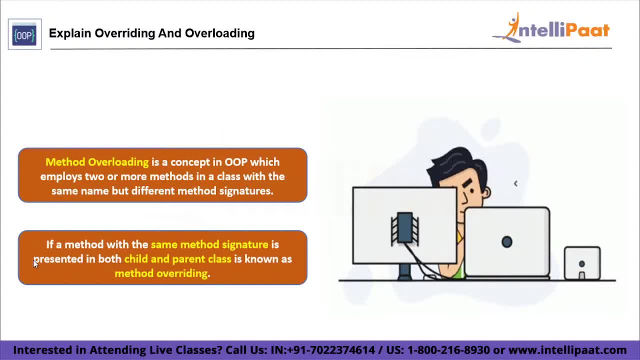 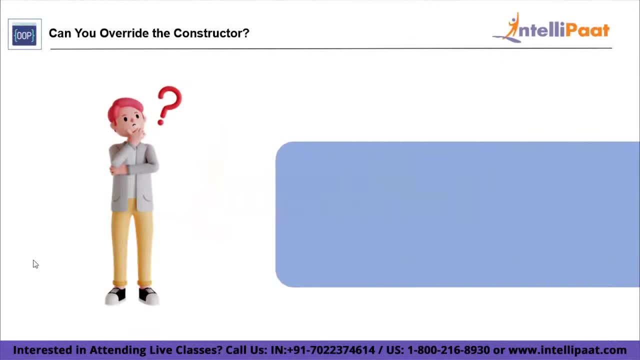 This is also known as runtime polymorphism as well. Now next question we have on our list is: can you override the constructor? Well, you cannot override the constructor, because it looks like a method, but it is not. It lacks a return type and shares the same name as a class. 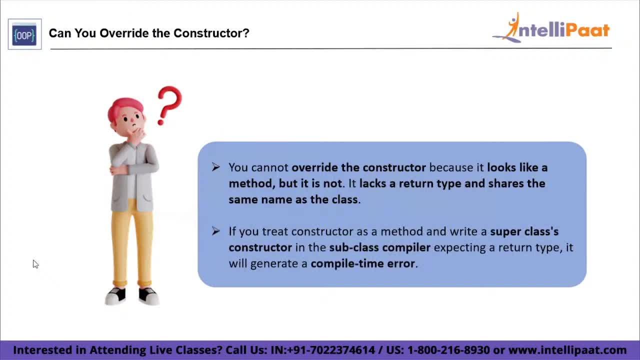 If you treat it as a method and write a superclass as constructor in the subclass compiler, expecting a return type will generate a compile time error, So you cannot actually override the constructor Now. finally, the last question on our list is if you have a class containing 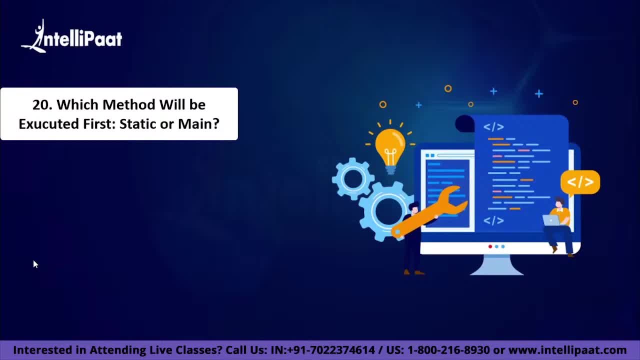 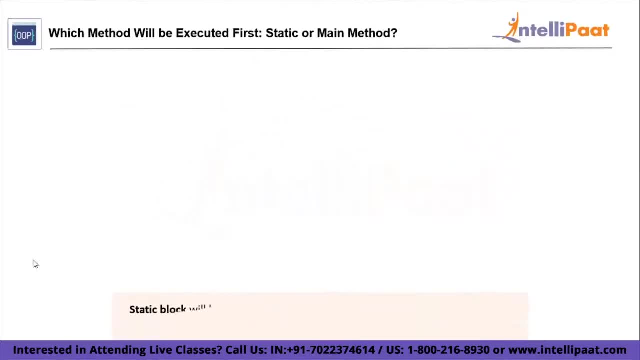 a static method and main method with the print statement. which print statement will be executed first? Now, this is a tricky question, but the answer to this is pretty straightforward. Many languages execute static block on priority basis. What it simply means is static block will be executed even before the compiler. 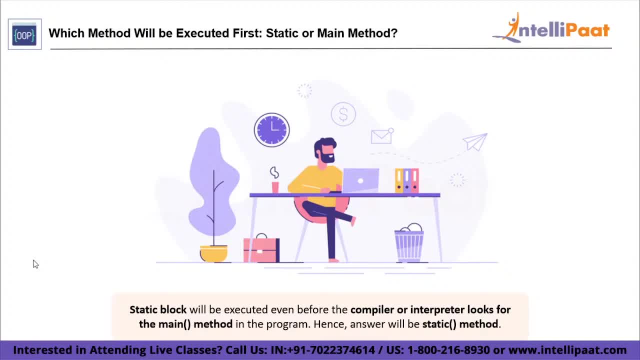 or interpreter looks for main method in program. Once the static method is executed, the main method will be compiled. Hence the answer to this question will be print statement and the static method will be executed first. That's all we have for this session. 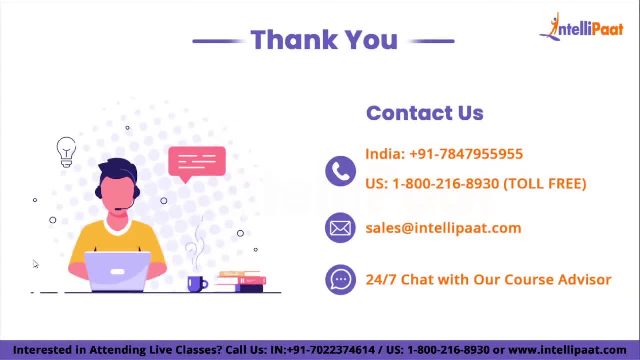 Thank you so much for being here till the end of this video. I wish you all very best in facing those technical interviews. If you want to come across more such technical videos or interview preparation tips, make sure that you hit that subscribe button below. 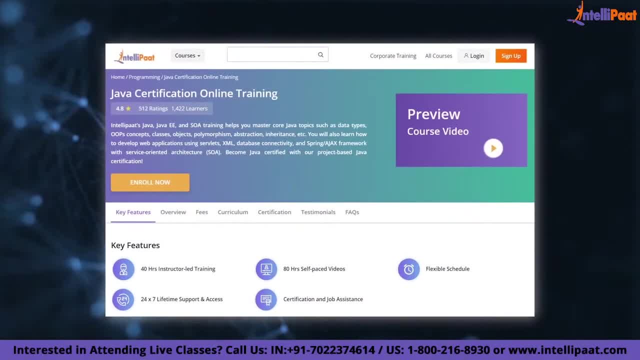 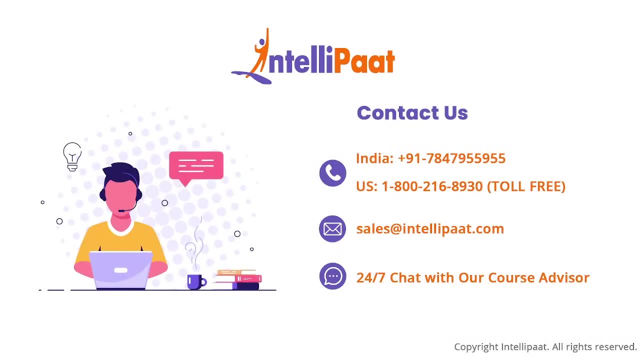 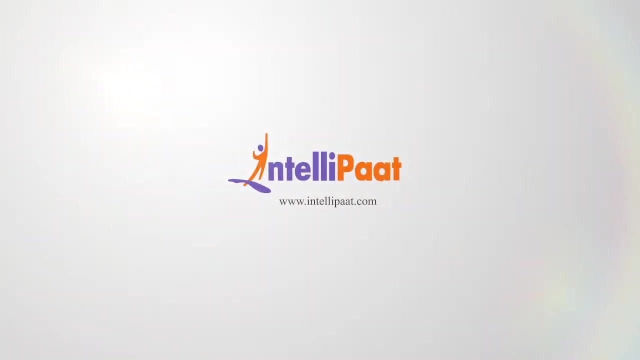 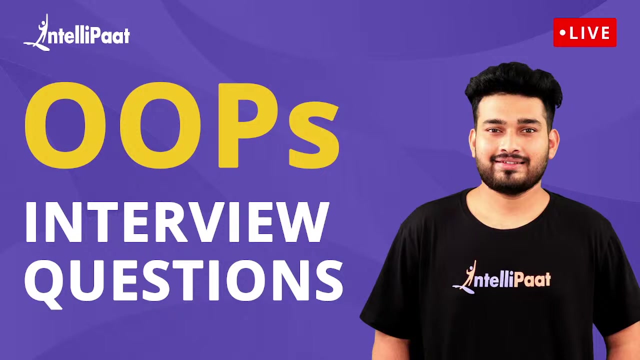 Just a quick info, guys. Intellipaat provides Java certification online training, mentored by industry experts, The course link of which is given in the description below. Thank you, See you next time, Bye, bye.